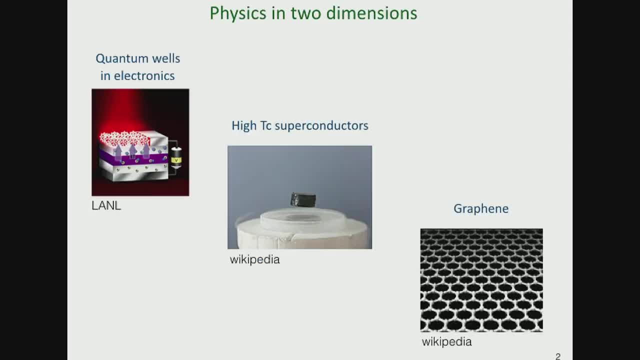 Tomorrow it will be two. OK, So let me start, And I start- by again speaking about two dimensions. This will be the topic of today, And, before going to fundamental physics, I would like first to say how important it is to understand what. 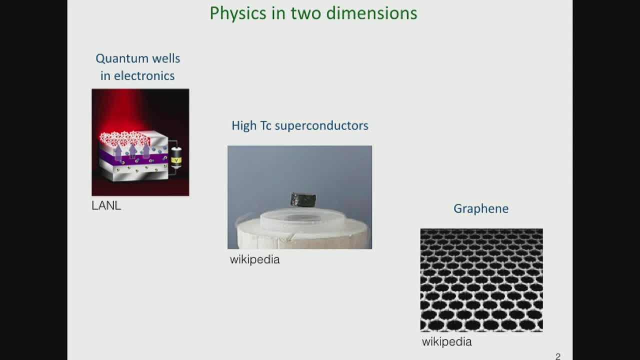 happens in two-dimension, how important it is from an applied point of view. There are many devices in our world, technological world now, which are based on two-dimensional physics, And here I have just given three of them, but there are many others. The three of them: 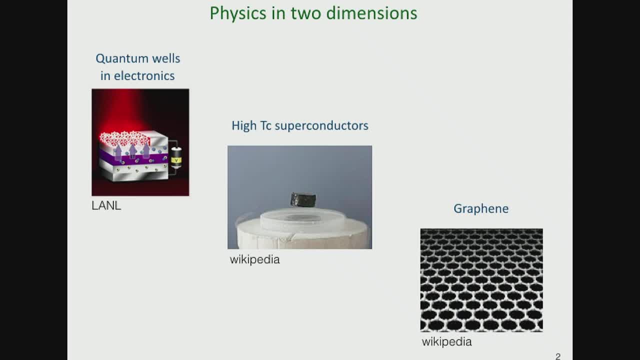 that I am pointing out. here are quantum wells, which are everywhere. They are becoming you in electronic devices, And a quantum well is nothing but a 2D gas of electron confined strongly by playing with semiconductors and with electric potentials. 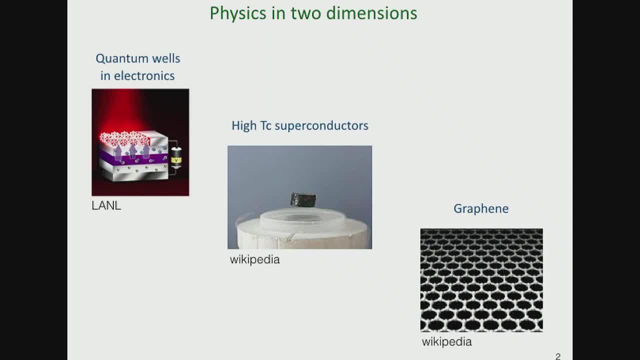 Another place where two-dimensional physics appears is in high-TC superconductor. It is now, I think, widely accepted that this superconductivity occurs because the Cooper pairs move in a two-dimensional environment, And another very famous example of 2D physics is graphene. 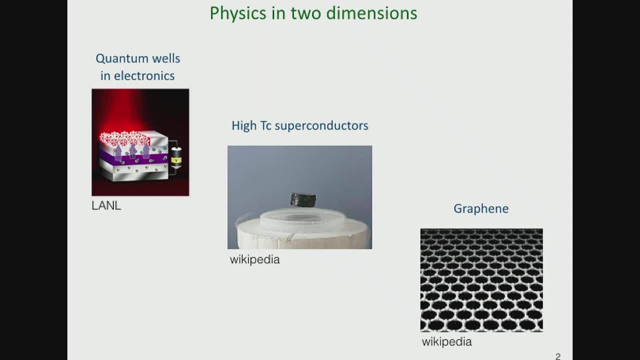 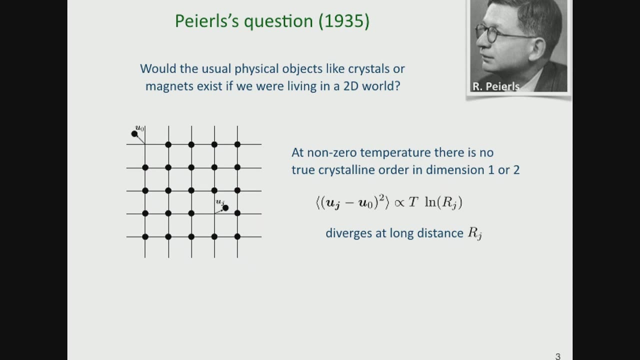 This set of carbon atoms, these sheets of carbon atoms which have very interesting properties for application. So this motivates to study two-dimensional physics. Now, there is also a fundamental motivation which is, as I mentioned yesterday, the fact that in 2D you do not expect 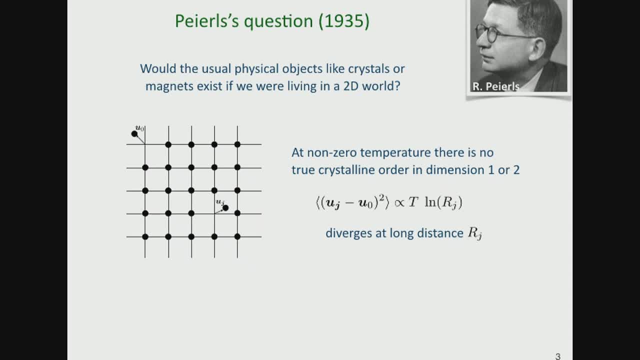 to have the same type of phase transition as in 3D, And this was understood first by Peierls in 1935.. And the question that Peierls was asking at that time was: if we live in a 2D world, would physical objects 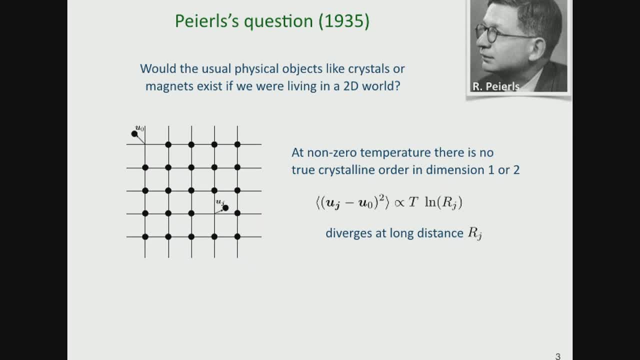 like crystals or magnets? would they exist? And the answer that Peierls wrote and that we will review thoroughly in the next slides is the following one: If you take a non-zero temperature, there is no true crystalline order in dimension one or two. 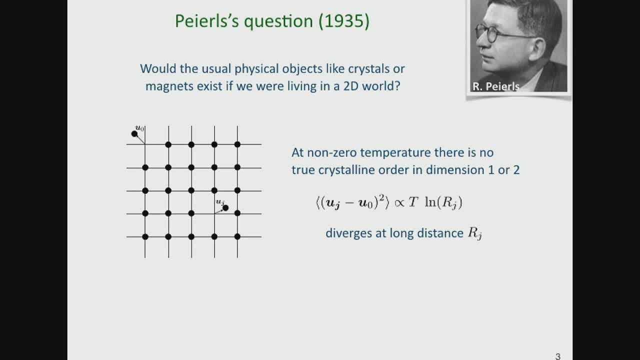 And the reason for that is that if you take a possible arrangement of a crystal, say a square lattice like that, if you look at the displacement of this atom that I labeled zero here I call this U0, this one I call it Uj. 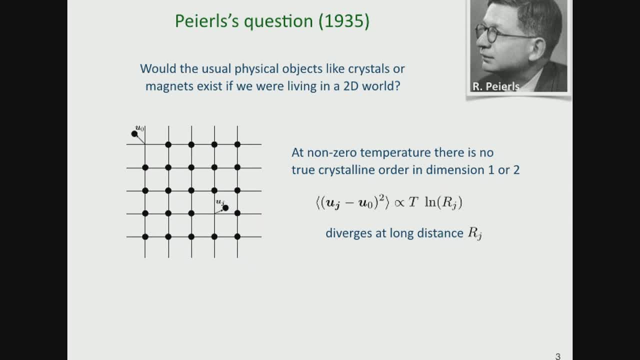 and I assume that I am at a non-zero temperature. so I look at the variance of the displacement of zero versus j, so Uj minus U0 squared and I average over thermal fluctuation. Then the result that you get in 2D. 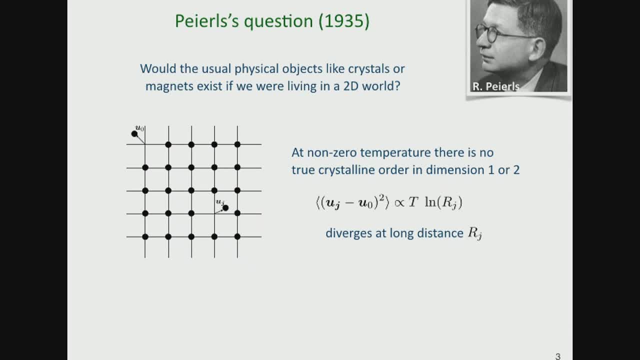 and again. we will show it rigorously in the following, but I am just announcing the result here. this variance is proportional: temperature times, the log of the distance between atom zero and atom j. This means that if I take Rj large enough, 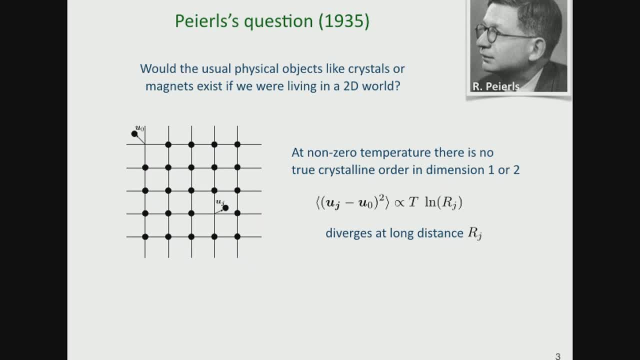 the log is going to tend to infinity and therefore, even if I know perfectly well where the atom zero stands, I will have no information where the atom j stands within a unit cell, because this quantity here will be larger than a square, where a is the. 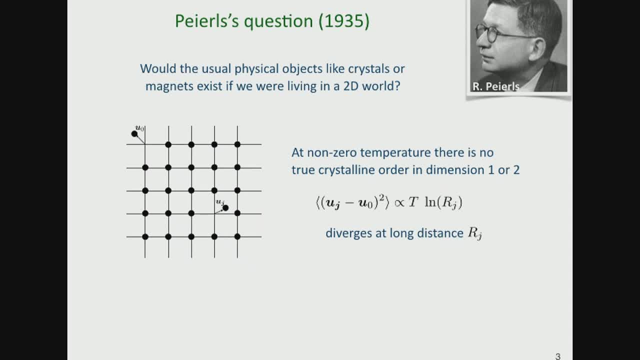 the size of the unit cell and therefore I will lose completely the long-range order. knowing where an atom is sitting, it doesn't give me an information where another atom far enough is sitting. okay, And this was understood, as I said, by Piers very early. 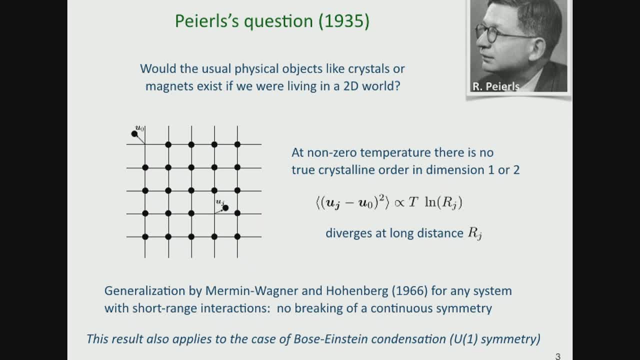 just after the beginning of quantum mechanics and it was generalized 30 years later by Mermin Wagner and Hohenberg for any system with short-range interaction. then this gentleman showed that you cannot have at a non-zero temperature. 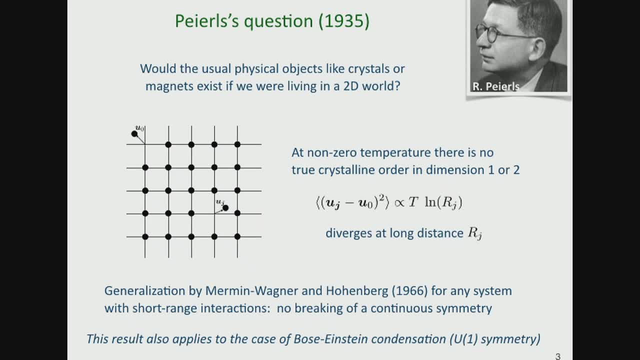 a phase transition involving a breaking of a continuous symmetry, the continuous symmetry here being simply the formation of a periodic lattice of atoms. And this, as we will see again today, also applies to the case of Bose-Einstein condensation, where the symmetry to be broken 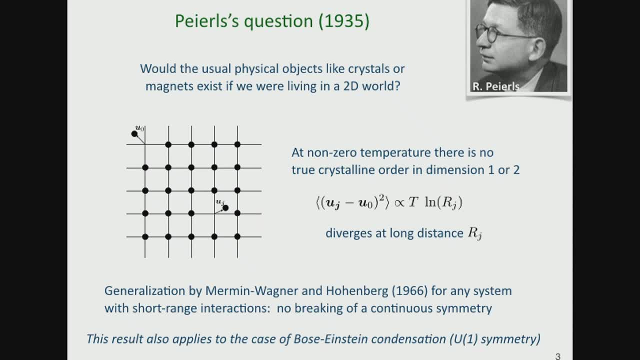 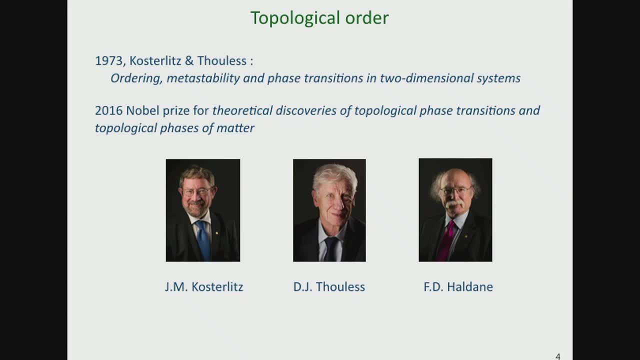 when you, when you both, condense a system in 3D, is that your macroscopic wave function acquires a definite phase. so you break the. you want symmetry for the phase. However, as I explained yesterday and I, which will be the topic of the two, two lectures- 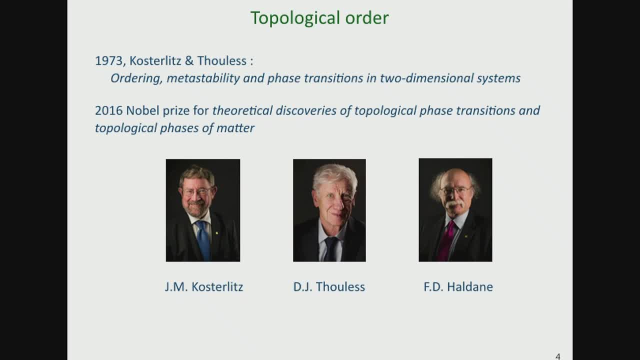 there is still room for unconventional phase transition, and this was understood by Kossel and Taules in 1973, in a famous paper which was called ordering, metastability and phase transition in two-dimensional systems. and last year Kossel and Taules got the Nobel Prize. 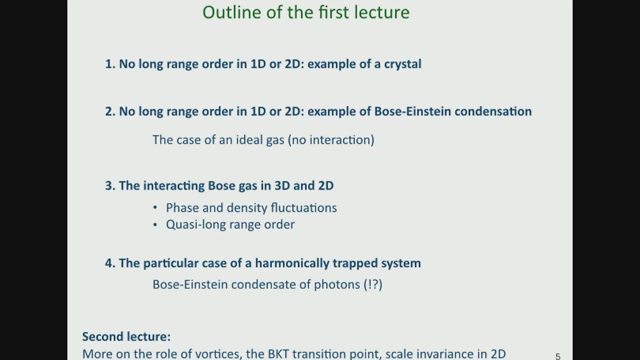 shared with Duncan and Haldane. So this is what we want to study. This is the outline of the lecture of today, So I would like to review the argument by Piers again. it may be something that some of you already know. 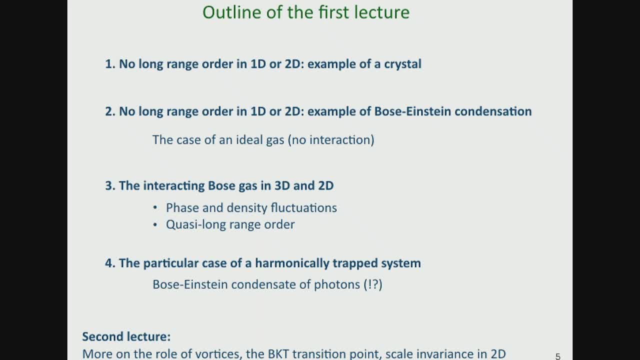 but I think it's good to see this kind of argument because it will play a role in the following. So I want to show that there is indeed no long-range order in 1D or 2D, and take the example of a crystal. 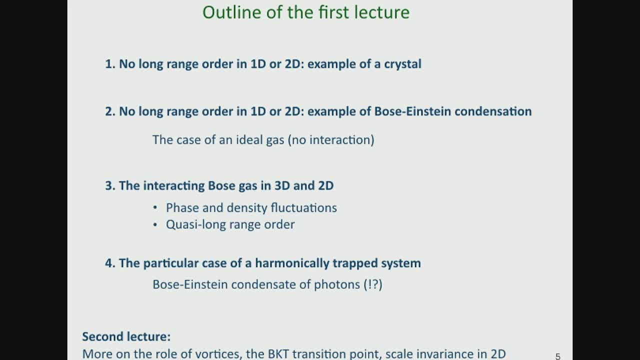 Then we will generalize this to the case of Bose-Einstein condensation, Again 1D or 2D. In the first part I will deal with an ideal gas-to-interaction and in the second part this may be after the lunch break. we will deal with an interactive gas-to-interaction. so this is an ideal gas-to-interaction and in the second part, this may be after the lunch break. we will deal with an interactive gas-to-interaction and in the second part, this may be after the lunch break. 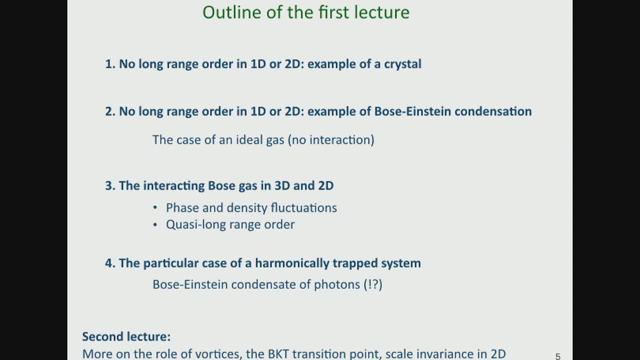 with an interacting Bose gas, where there we will be more careful by separating what is called phase fluctuation and density fluctuation, and we'll show actually that interactions bring some new features with respect to ideal systems, because it brings this idea of a quasi-long-range order. 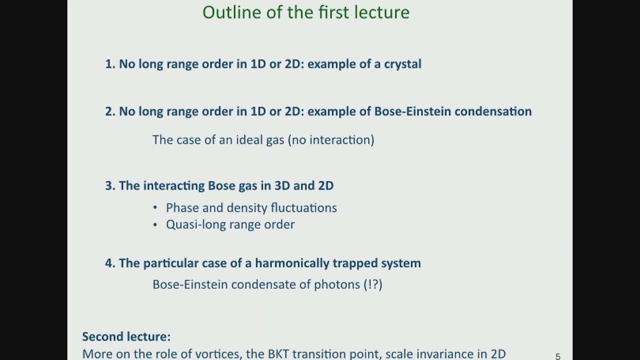 not the true long-range order, which is forbidden because of the Mermin-Wagner theorem, but quasi-long-range order. And I will finish the lecture of today by discussing the case of a harmonic electrop system and speak of something which at first sight looks very strange. 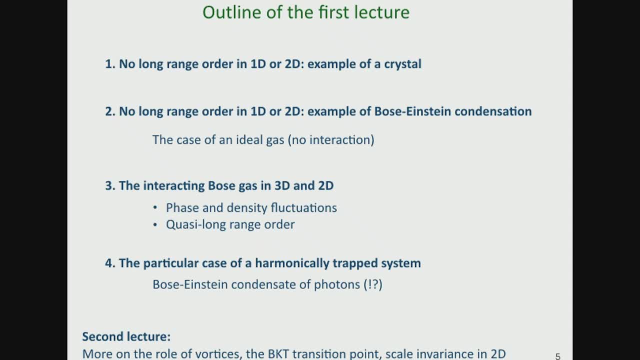 which is the case of a harmonic electrop system, and speak of something which at first sight looks very strange, which is the Bose-Einstein condensation of photons. but I will try to convince you that this is indeed possible and has been seen experimentally. 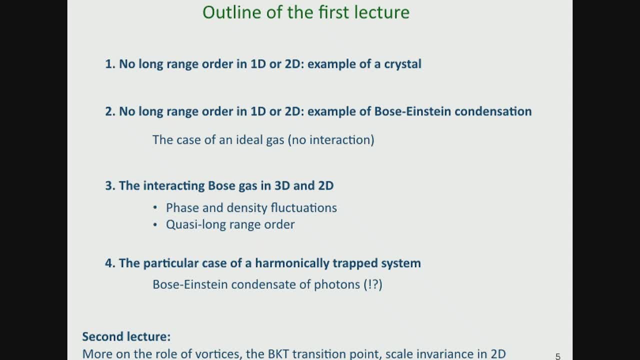 And tomorrow, in the lecture of tomorrow, we will learn more about the role of vortices and we will really understand the BKT transition point, and I will discuss a nice feature that occurs in two dimensions, which is not present in 3D. 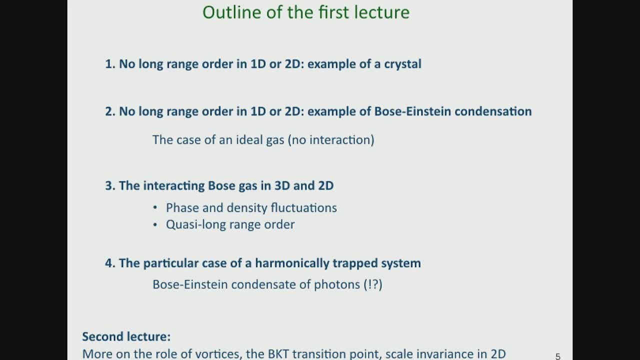 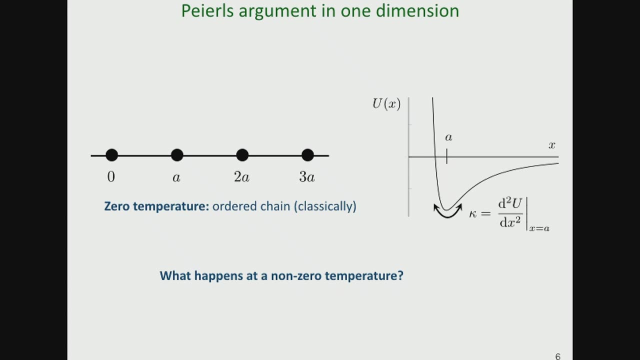 which is the notion of scaling variance. So let's start with today's lecture And this argument by Peierls that indeed there is no long-range order in 1D or 2D. So the argument of Peierls, let's start with one dimension, where it is the simplest. 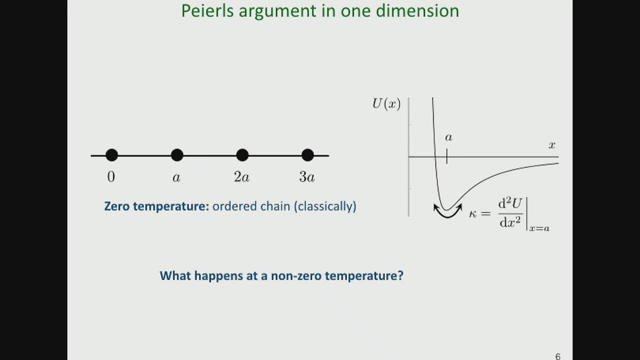 the argument of Peierls goes in the following way: Let's suppose that I have my atoms which are interacting by some short-range interaction, and I model this short-range interaction by a potential u of x, which is, like this, so attractive at a long tail, which is attractive for a long distance. 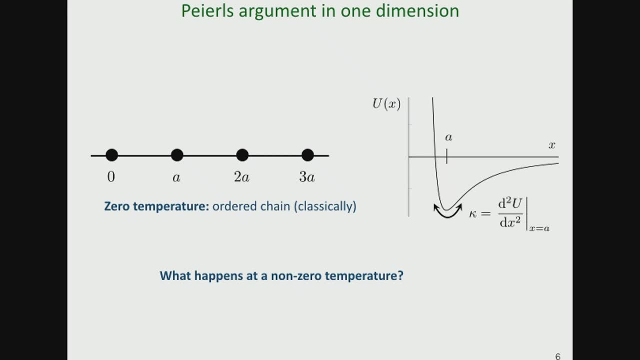 a local minimum, well, a minimum here for distance a and then a short-range repulsion. So if I am at temperature zero, it's clear that all atoms will make a perfect crystal, classically, and the distance between the two atoms will be equal to the two little a, where a is the position of this minimum. 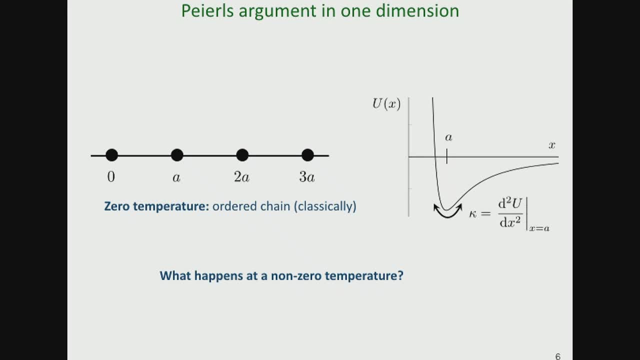 Okay, so at zero temperature, classically, there is no fluctuation. the answer is easy. If it was a quantum description, then I would have quantum fluctuation and it would be a bit more difficult. but let's do it classically for the moment. 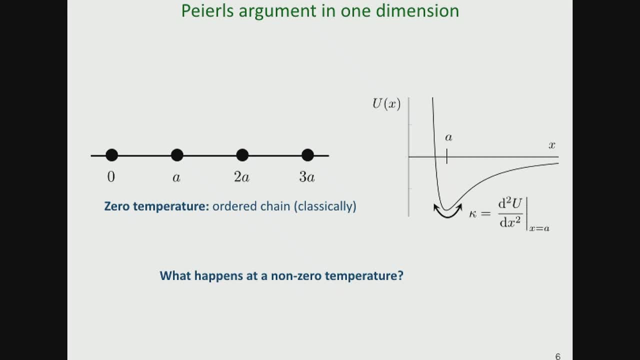 So I expect a perfect crystal at zero temperature. What happens at non-zero temperature? So I will excite some fluctuations because of thermal fluctuation, and this fluctuation will be characterized by the spring constant here If I replace this by an approximation, which is the parabolic potential. 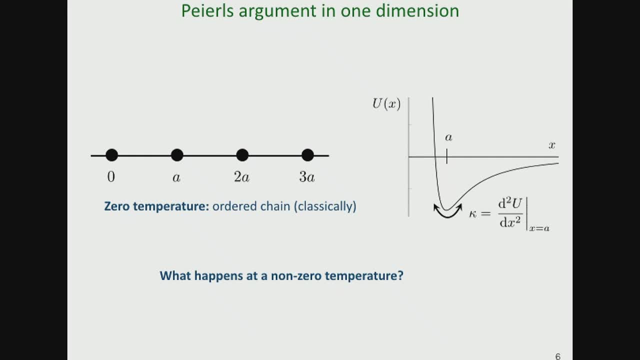 I have the strength of the oscillator is this: kappa, which is the second derivative of u with respect to x. taken in, x equal a. So I will now model my change. So I have my chain at a non-zero temperature and the best way to do that is to use periodic boundary conditions. 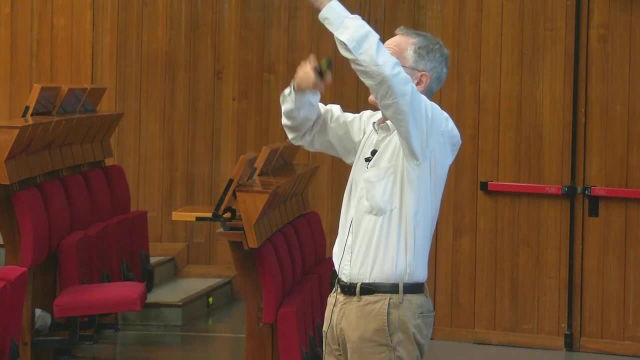 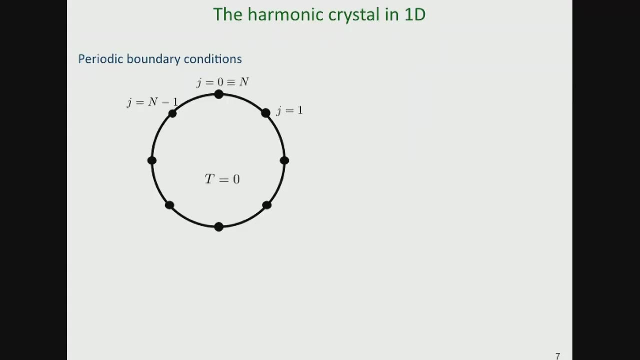 So, instead of having a chain which is between minus infinity to plus infinity, I put my particle on the circle and I put n particle for a circle which has a length n times a. So at temperature zero again, I have one atom every a. everything is perfect. 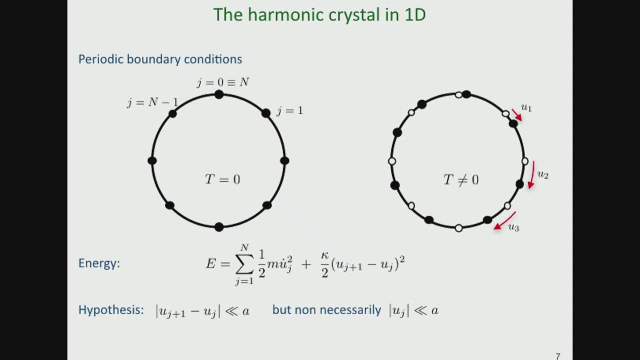 Now, if I'm at non-zero temperature, the atom one may move by a quantity u1,, the atom two may move by a quantity u2, and so on. And if I look at the energy of this system, I have both some kinetic energy and some potential energy. 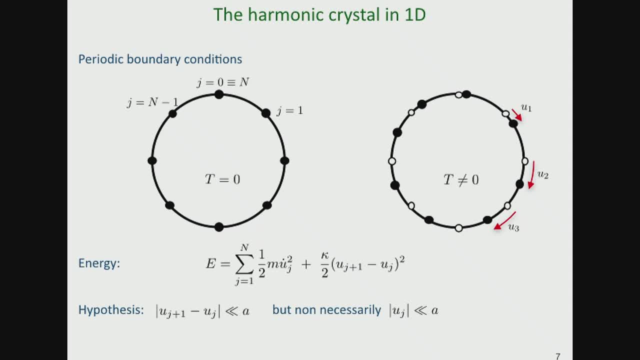 due to the interaction of the atom between the atoms, And so the kinetic energy is here. it's proportional to the uj square. So uj again is a displacement with respect to the equilibrium position And the potential energy is just the proportion. 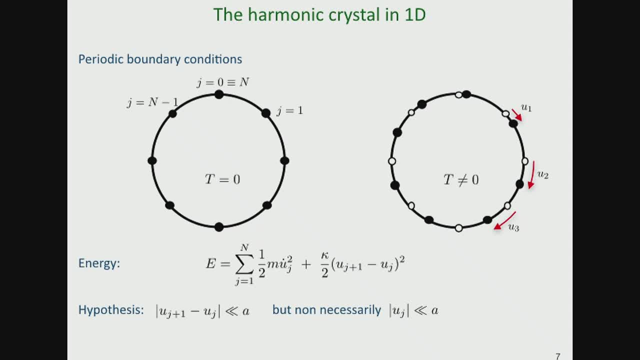 So this is the distance between the atom one and atom two, atom two and atom three, And it would be minimum if the distance would be a, and if the distance is not strictly a, it's proportional to the square of the uj plus one, the displacement of atom j plus one minus uj square. 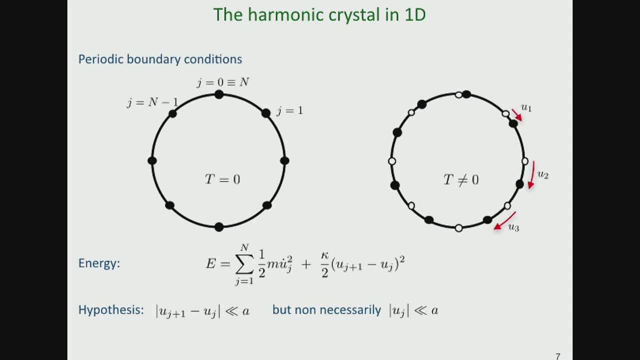 and all this is sum over j, And the hypothesis here is that I am allowed to expand the potential between the atoms. so uj plus one minus uj has to be small compared to a. But I don't assume that uj is small compared to a. 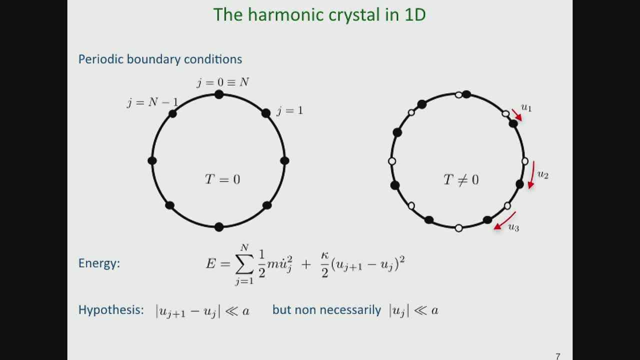 That is the atom. j may move by a lot as long as its neighbors move by nearly the same amount. So this is the hypothesis. So how does one treat that? Well, I suppose that you have all seen this in your lecture. 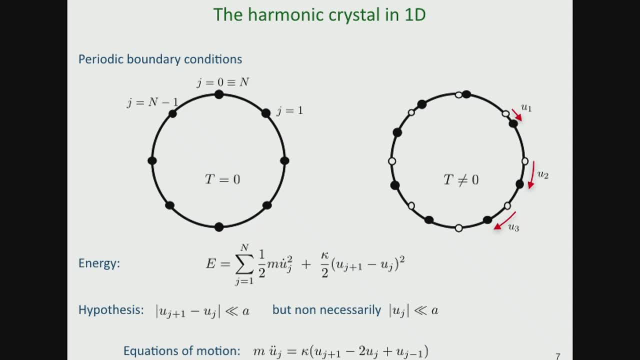 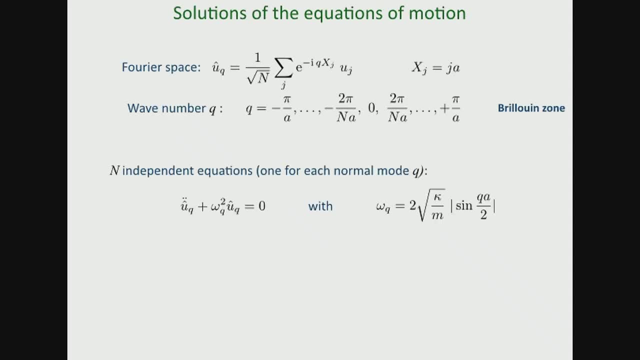 You can write the equation of motion for the variable uj and uj double dot, double time derivative is coupled to itself and to the two neighbors j plus one and j minus one. And a simple way to solve this equation. 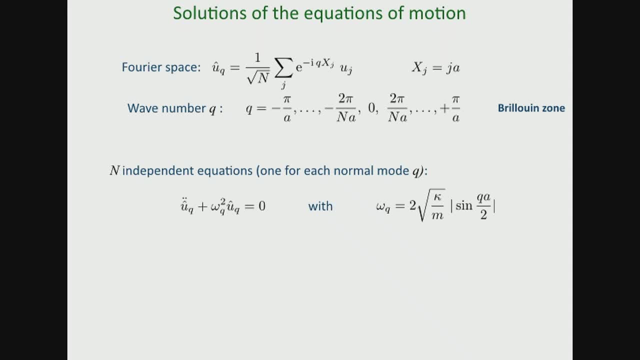 excuse me, is to go to Fourier space, to Fourier transform the equation. So I introduce q with a hat, which is just the Fourier transform of uj. So q is a wave number here that I chose in the Brillouin zone. 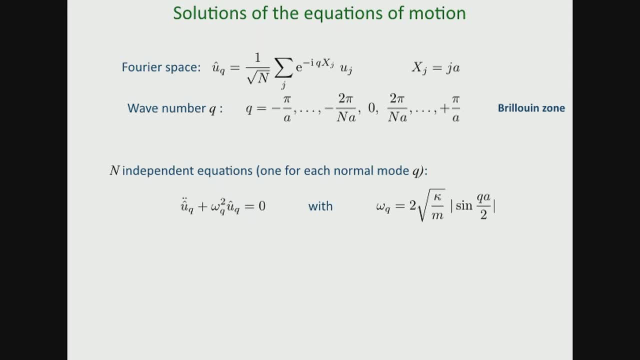 Emmanuel has described this in his lecture so I'm not going through that in detail. but q goes from minus pi over a to plus pi over a, And when you are in Fourier space you get normal modes and you get n independent equations if you have n atoms. 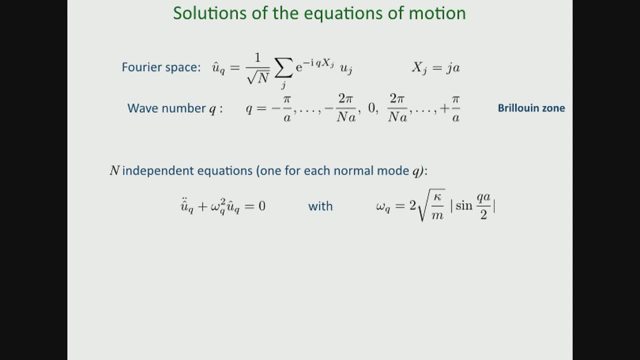 and each equation you write: uq, double dot plus omega q square uq equals zero, where the frequency of the mode q is just given, well, by sine qa. so again, the wave number here times a coefficient which involves the spring constant. 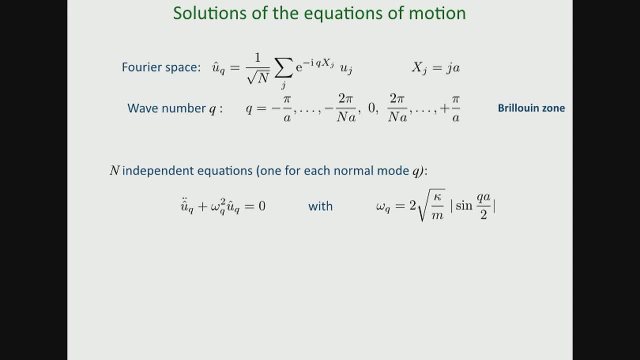 and the mass of an atom. So again, this is something I think you have all seen once, so I'm going pretty fast, but if you have any questions, as for the other speakers, don't hesitate to raise your hand. At this stage, I suppose everyone is happy. 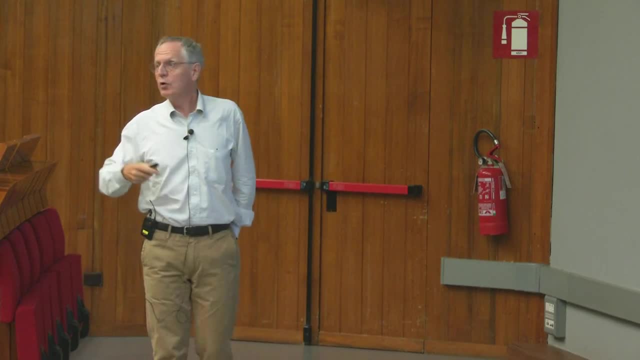 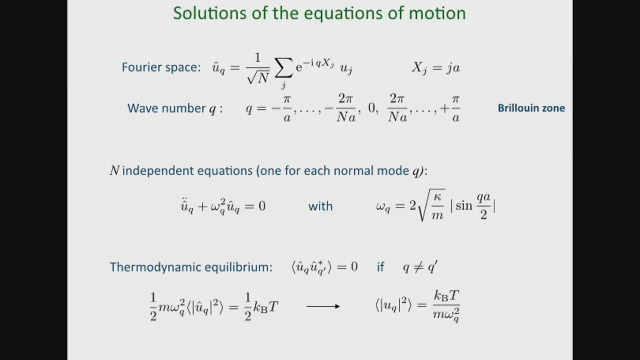 Yes, Okay. So then we look for thermal equilibrium for this system. So we have n independent harmonic oscillator, because this is the equation of an harmonic oscillator. so at thermodynamic equilibrium a given oscillator is decoupled from the other, because they are independent. 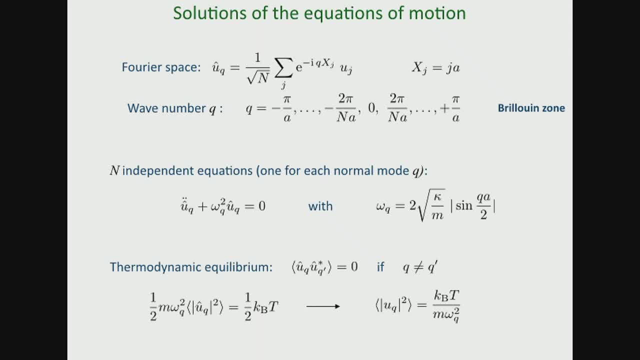 their equation is not coupled. so I know that the average of uq uq prime will be zero if q is not equal to q prime. and if I take q equal to q prime in this equation, then I have the equipartition of energy. 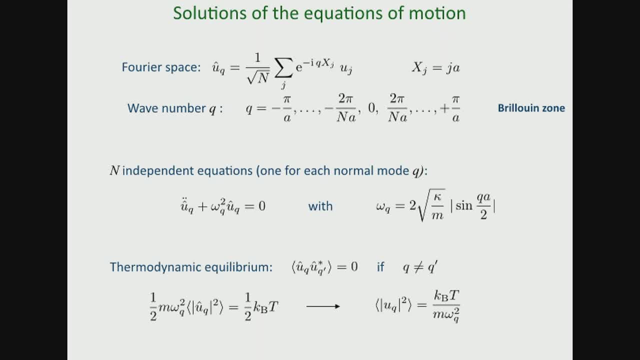 because I'm doing classical statistical physics. so one half of m, omega, q square, uq square, is just equal to one half kt, which tells me that uq square is proportional to kt. This is the important result that actually will be valid even in 2D or 3D. 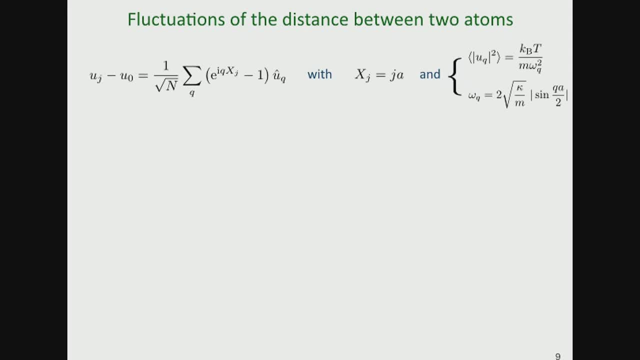 So now let's go back to the problem that Piers had risen. Let's look at the fluctuation of the distance between two atoms. So I take the atom 0, which moves by a quantity u0 because of fluctuation. I take the atom j, which moves by a quantity uj. 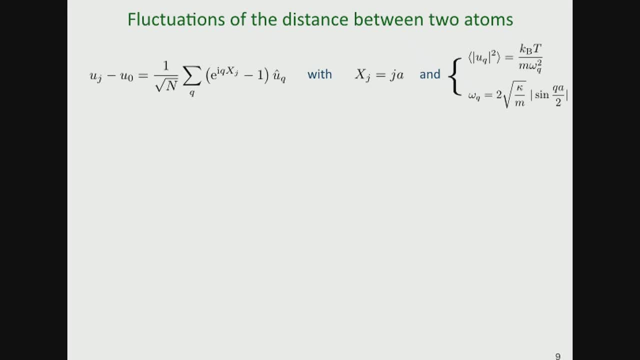 and I look at this quantity: uj minus u0,. I plug here the Fourier expansion that I had written before, where xj, here is the position of the atom j, the atom 0 is in position 0, so I've got a 1 here. 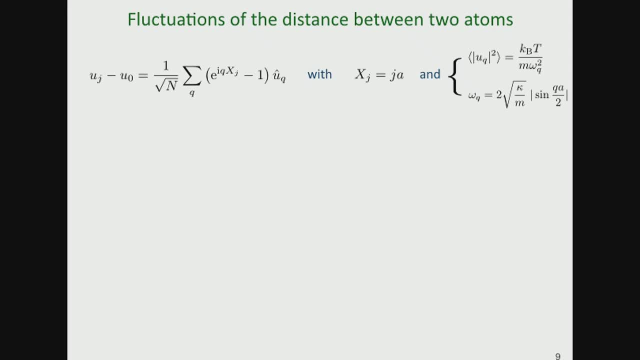 and I remind you that now I have to take the thermal average of this, knowing that uq square is proportional to temperature. it involves a frequency, omega q, and this omega q is itself proportional to sine q of a sine qa. So here, 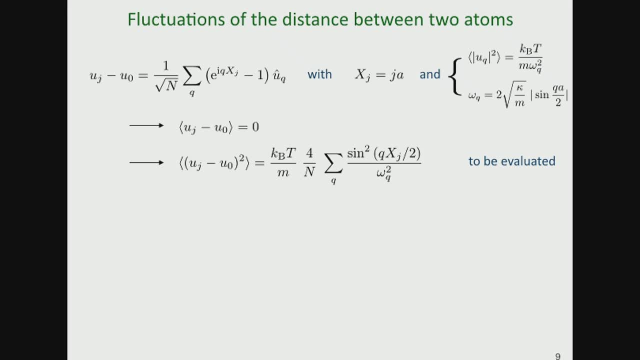 I take the square of this. well, first I look at the average value of the quantity itself. but this is going to be 0 because all the uqs are 0 in average. so in average the atom stays at the position. I am interested in the fluctuation. 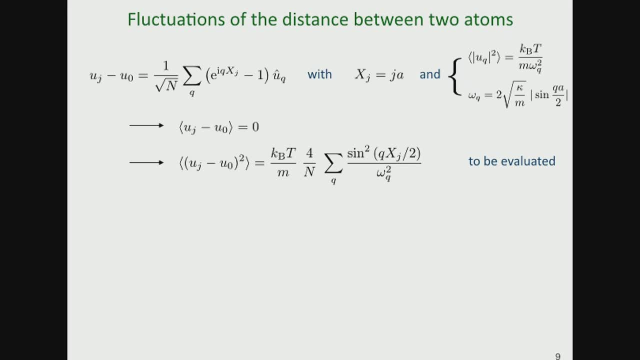 so I take the square now and I take the thermal average, which is this kbt over m, which is here, and I am left with the sum of all modes of the system of sine square of qxj over 2 divided by this frequency. 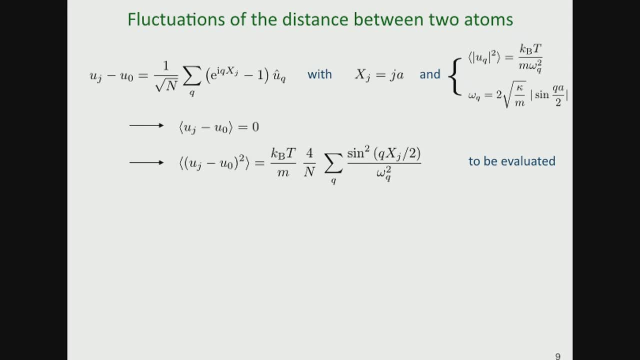 omega q square. This is what needs to be evaluated And this is when evaluating that that we will see whether Pi-R is correct and how one goes from 1D to 2D to 3D. So, in order to evaluate this, 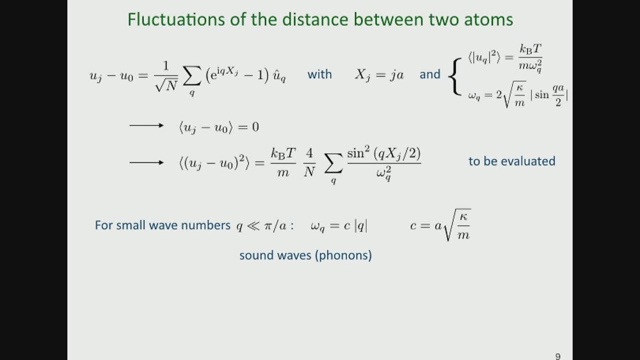 I am going to make an approximation, which will be validated later on. I will assume that the physics of low dimension, the physics of Berensky, is dominated by low momentum or, if you prefer, large wavelengths, and you will see why it is like this. 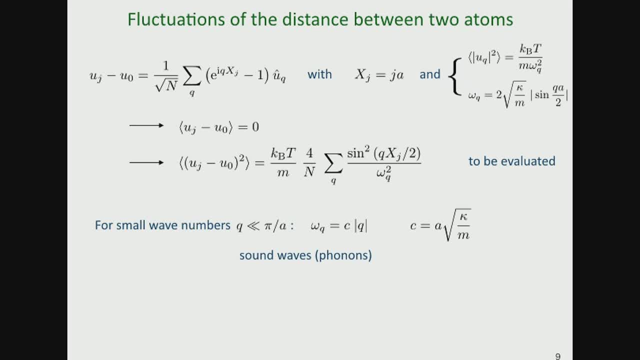 in a moment. So if q is, I can assume that q is small. then it simplifies the algebra. I can say that q is small compared to Pi over a, which means that I can linearize the sign here and I get simply omega q proportional to q. 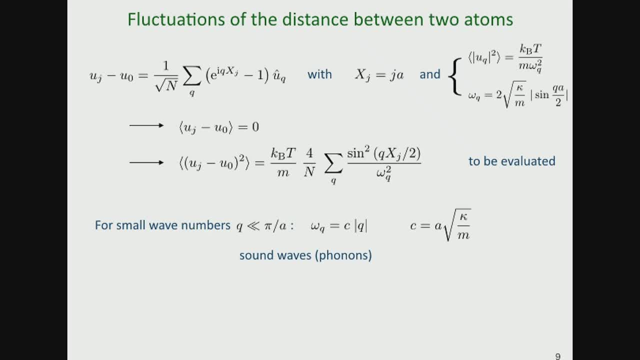 which just means that I am looking here at phonons, at sound waves only, and these are the excitations which dominate the physics. Ok, so the omega q square which is here, I will replace it by cq square, and the second step that I have to do: 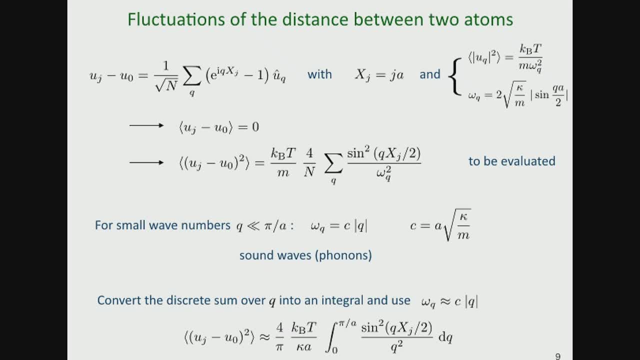 is to replace this discrete sum, which are never easy to evaluate, by an integral, and the integral over q here runs from 0 to the maximal value of q, which is Pi over a. so I get here in the integral, this sine square which is not modified. 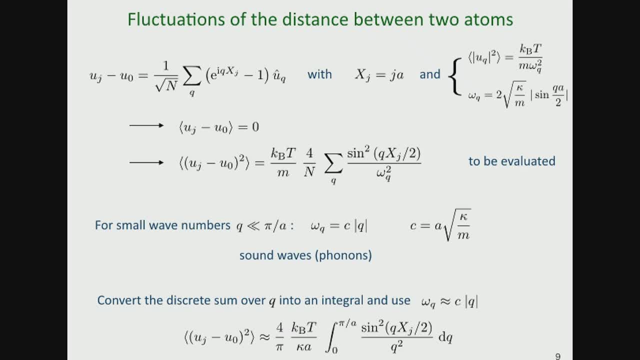 and the omega q square which I had here, which has been replaced by q, so I get a q square in the denominator. So keep this in mind, because this is really the structure that I will discuss both in 1D, 2D and 3D. 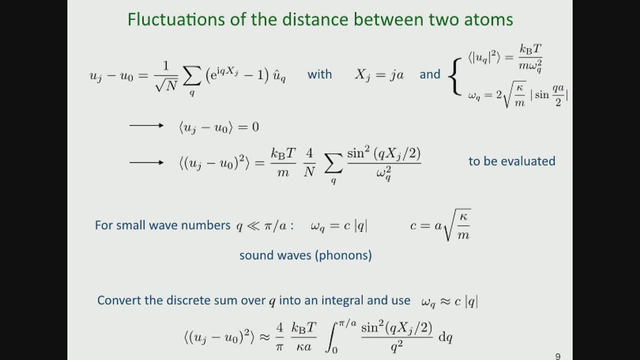 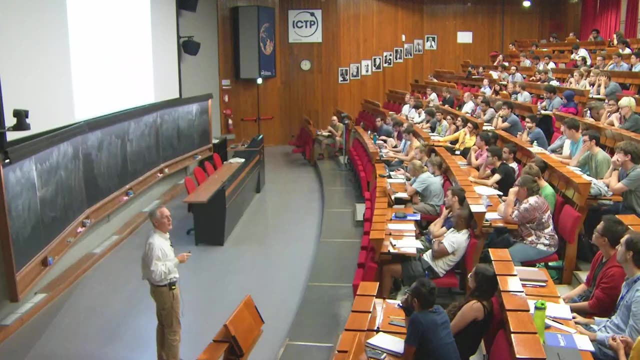 And the coefficient which is in front is kbt over something which involves the parameters of the problem, the spring, constant, kappa and the distance between two sides. little a, Ok. so let's try to evaluate that. if there are no questions at this stage, No. 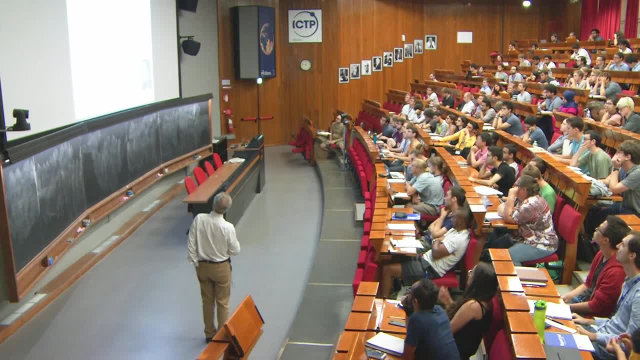 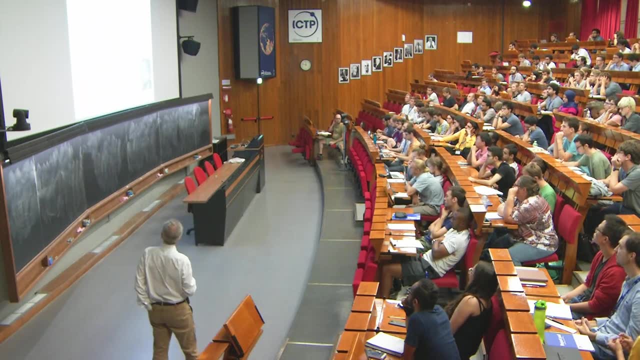 Let's try to evaluate that. So it's an integral. so if I, if I replace the upper bound by infinity, actually I can calculate the integral exactly and the result that I get in 1D for this integral is something which is kbt again. 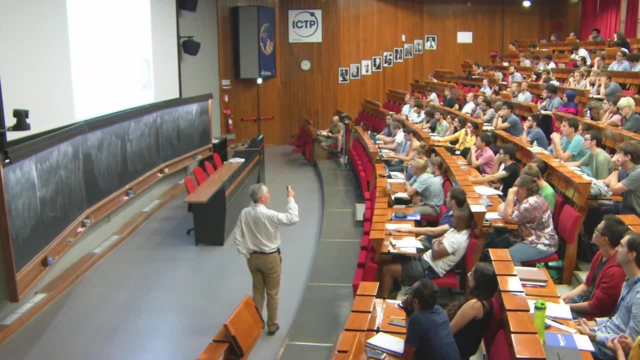 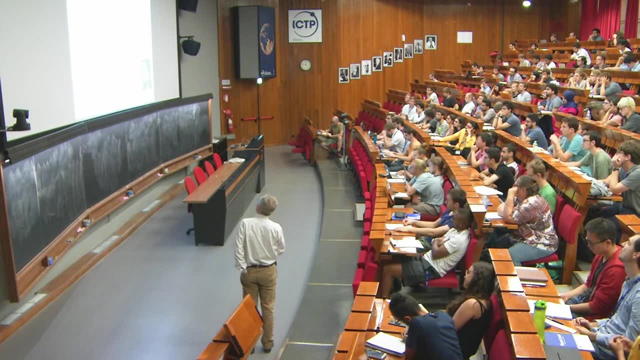 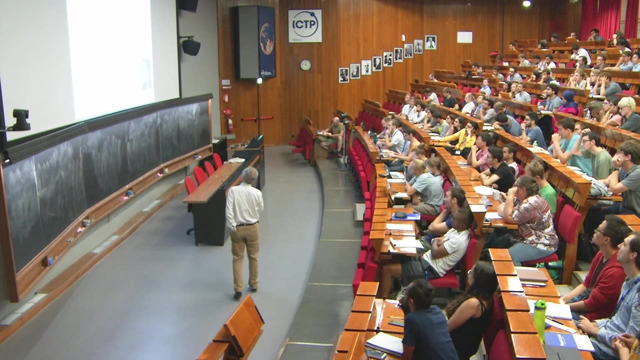 this was proportional and the integral of sine square over x over x square integral from 0 to infinity is equal to Pi over 2. so I get finally this result here and I get the fact that first I can look where are the modes which contribute the most here and I get 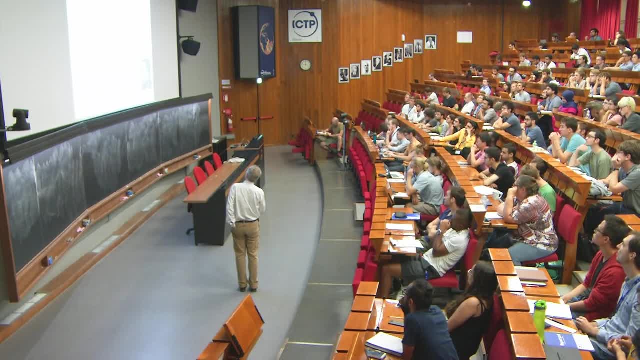 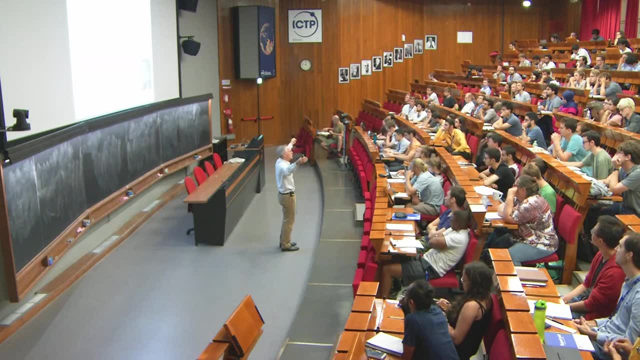 from this integral that the modes which contribute the most are the q on the order of Pi divided by xj. that is, if I take my two atoms, one atom in 0, one atom in j- the modes which contribute the most to the fluctuation. 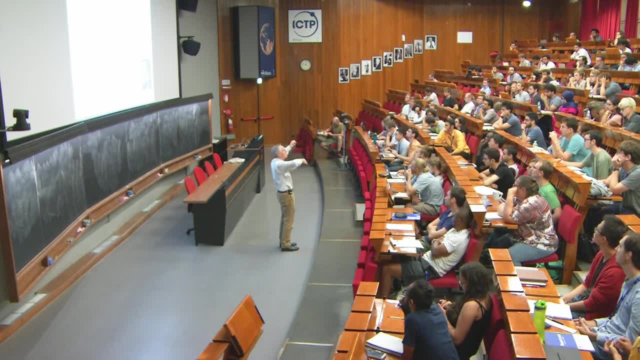 of the distance between these two atoms are the modes which have a wavelength on the order of this distance. Ok, so, since I'm interested in long distance behaviour, indeed, these modes have a very low q. this validates the approximation that I was looking at only sound waves. 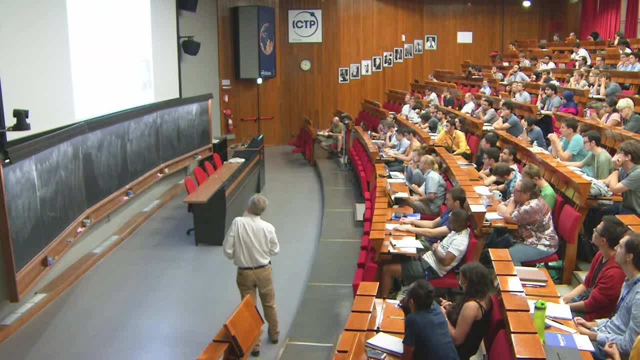 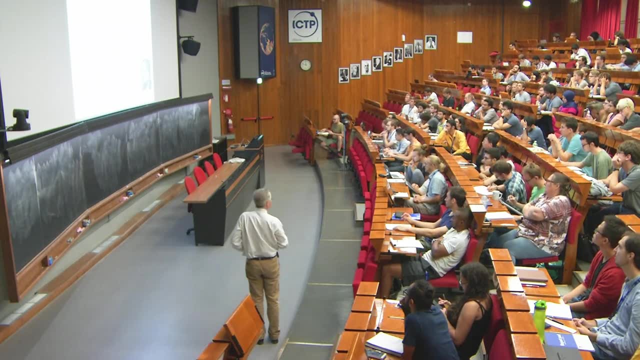 And more important, and again, this is what Peierls showed. when you look at that, you see that this function here will get larger and larger when xj gets larger and larger, which is what I said before. that is even if I know perfectly well. 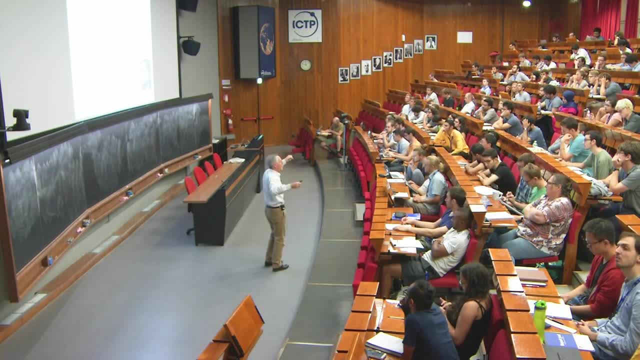 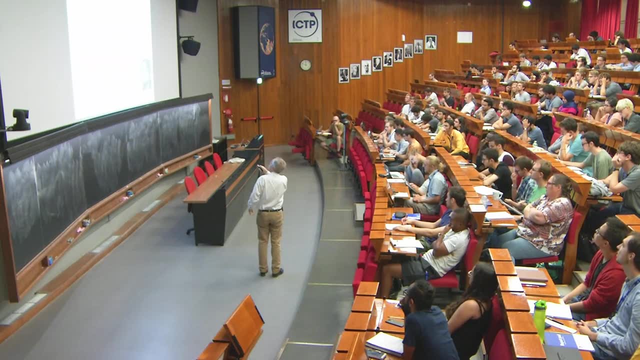 where the atom 0 is sitting. I know perfectly the value of 0. if I take j far enough, I will have no information where the atom j is sitting within a lattice spacing, because this whole quantity here will be larger than little a or little a square. so I don't. 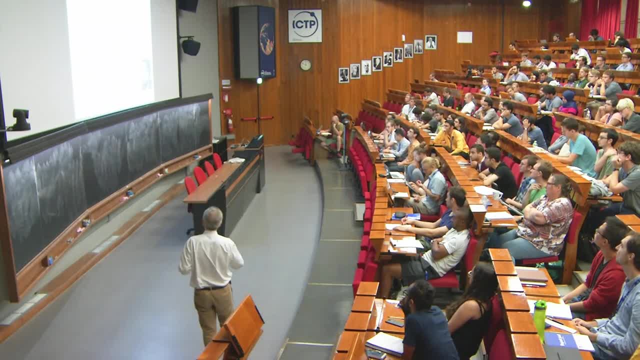 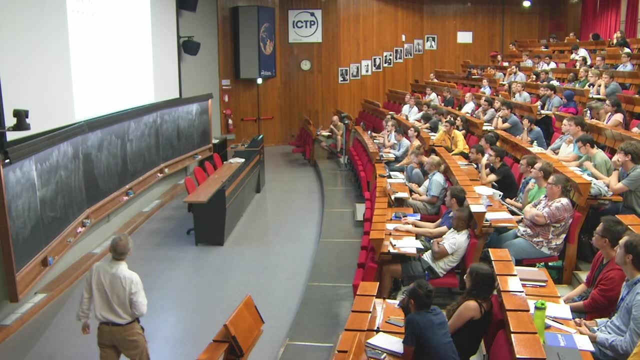 will not have a true crystal. I will not have any long range order. No long range order in 1D at non-zero temperature. Is that clear for everyone? Ok, So what about 2D now? So in 2D you can do exactly. 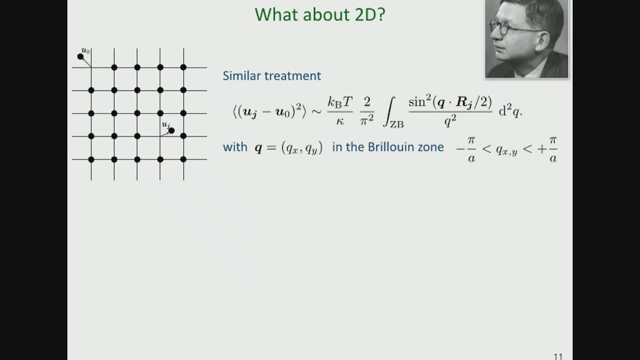 the same treatment. It's a bit more complicated from a purely technical point of view because in 1D I was. since I had only one dimension, my atoms had to move along this direction. but now in 2D, the atom may move in this direction or that one. 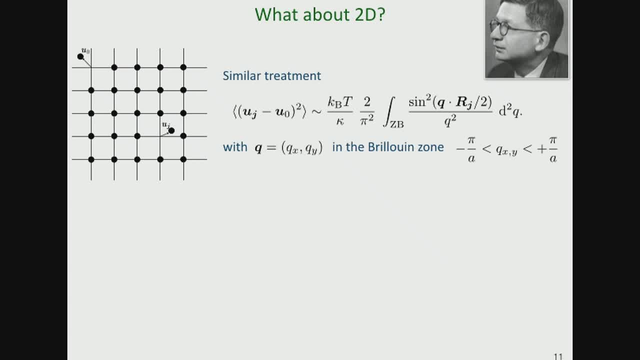 so I have to. when I look at the sound waves I have to look at the so-called polarization of the sound wave, the orientation of the motion of the atom. so technically it's a bit more complicated. but here I'm not so much interested in the technical details, I just 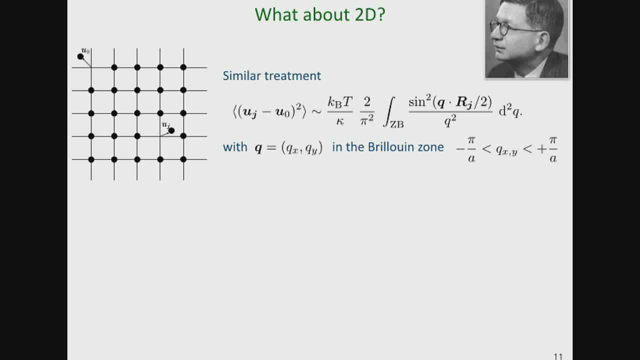 want to look at the global structure of the result, and the global structure of the result will be exactly the same as in 1D, that is, I will still get, when I calculate the displacement, the variance of the displacement of uj minus u0 here. 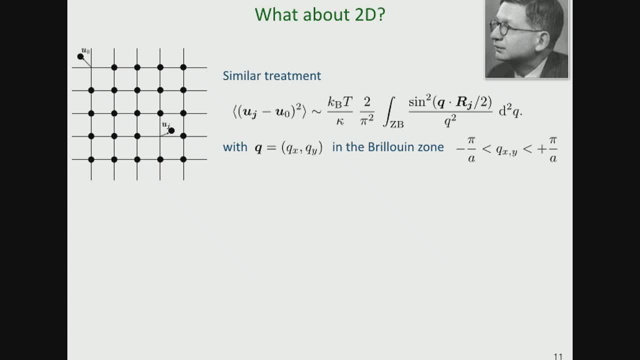 I will still get something proportional to the KBT. I will still get an integral of the Brillouin zone, which is now not a segment but it is now a square which goes between minus pi over a and pi over a, with qx and qy, and in the integral, 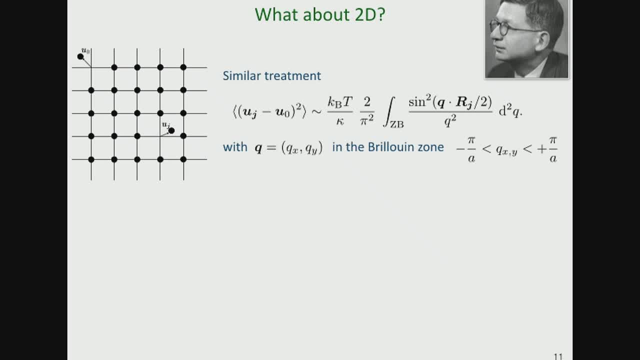 as before, I have a sine square of q times the distance between the two atoms I'm considering, divided by q square- because again I'm looking at sound wave- and now integrate not over a single dimension of q but over dqx and dqy, because I am in 2D. 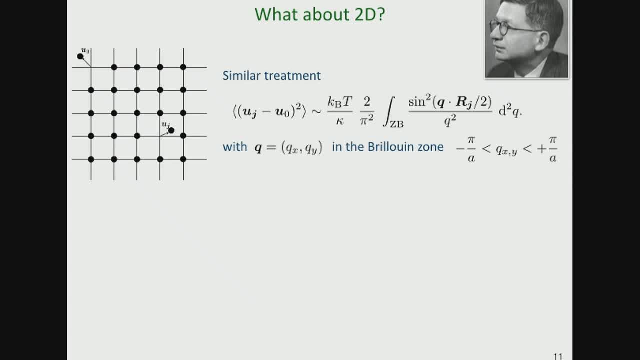 so the only difference at this stage is these two here telling me that I have to integrate over two directions and not one, but this is enough to already change a lot of the physics with respect to 1D. indeed, when you want to calculate this integral, so I can. 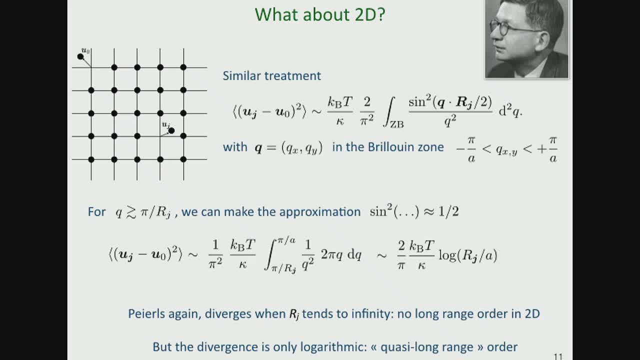 in 1D I could calculate it exactly in 2D. I have to make some approximation. so an approximation that I can do- if I assume that I am restricting myself to q on the order of pi over rj or larger- is to replace the sine square by: 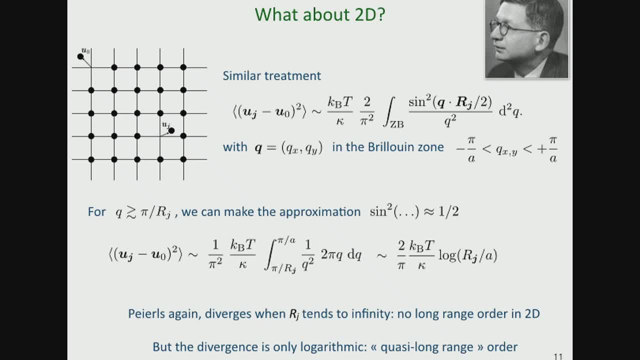 one half. I could do something more precise, but at this stage I can do that to get a rapid result. so I replace the sine square by one half. so this: get rid of these two here, and I'm left with 1 over q square times d2q. 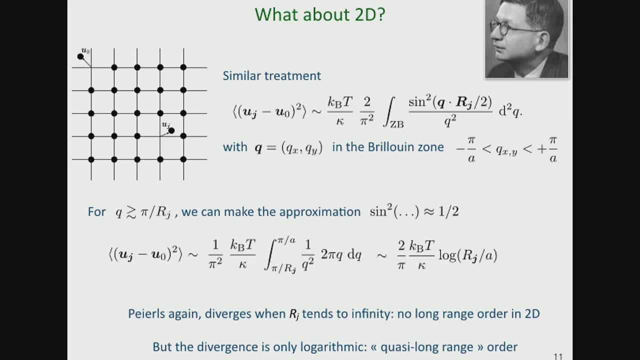 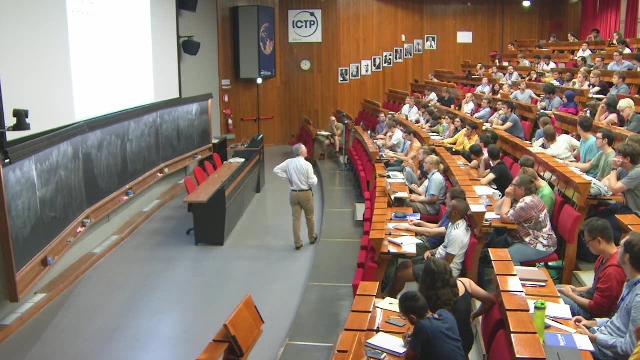 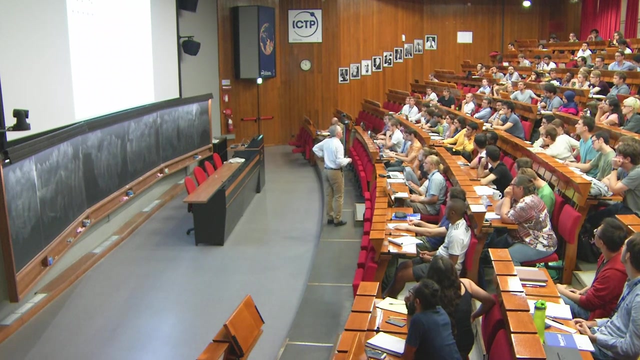 d2q is the element of surface in the Brillouin zone. so it's, if I take polar coordinates, this is 2 pi q, dq and 2 pi q. yes, you have a question, of course it's. what is that that? so I look at the displacement. 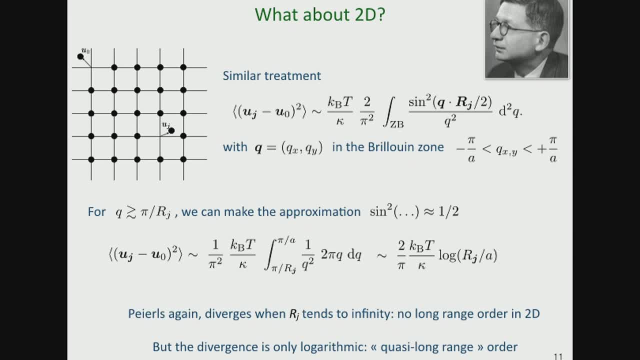 of the atom j with respect to the equilibrium position. I call it uj. I look at the displacement of u0. it's not rj, it's a displacement with respect to the equilibrium position. thanks for clarifying this. and so here I get, because I'm in 2d. 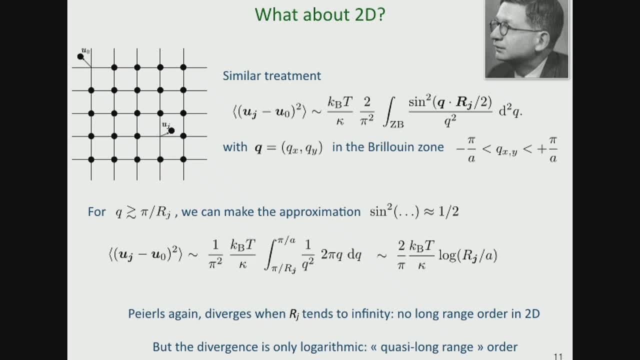 I get in polar coordinates 2, pi, q, dq, and so I'm left with an integral over q which goes: I have the 1 over q square times q, so I have 1 over q, and the integral of 1 over q is a log. so I get log of the upper bound. 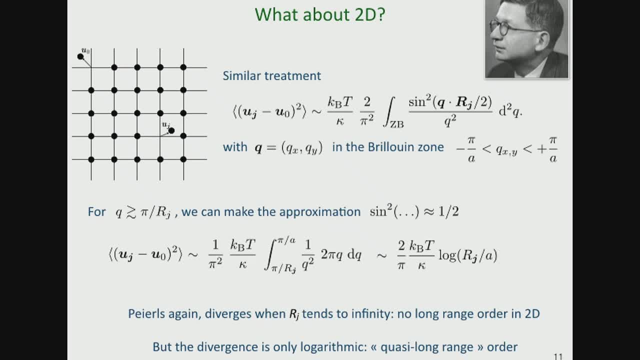 divided by the lower bound. the upper bound is pi over a. pi over rj is the wave vector q, for which the smallest wave vector q, for which this approximation holds. and then I'm left with this log of rj over a, and this is the result I was announcing at the beginning. 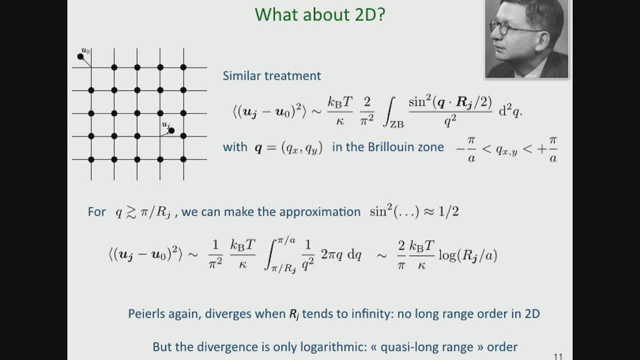 this variance of the displacement with respect to the equilibrium of j minus 0 here is proportional to temperature t and varies logarithmically with the distance rj, which means that, again, if I take a very large, even if I know perfectly well the value of u0. 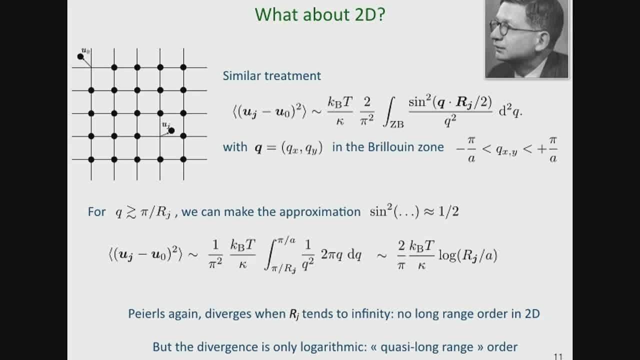 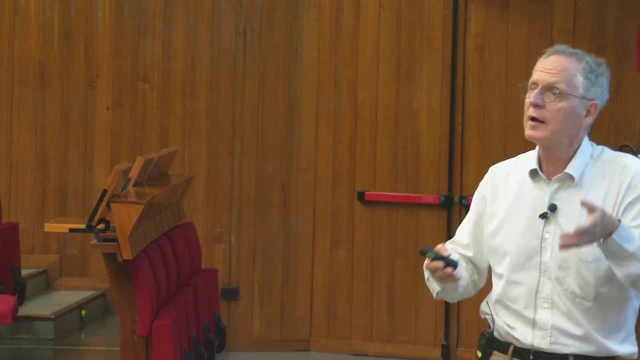 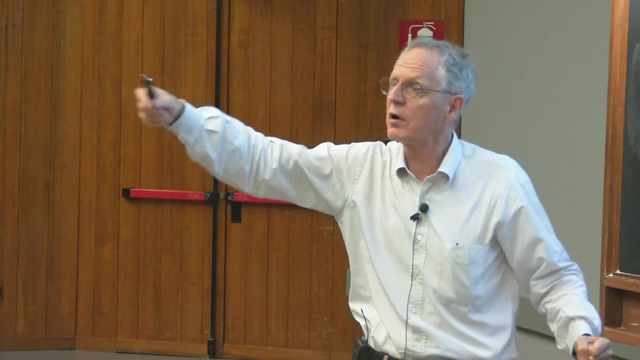 the value of uj will not be defined within better than little a, so I will not know actually where the atom j sits within a unit cell. so again, I do not have long range order. that is, knowing where an atom in the crystal is not enough to know where all the other. 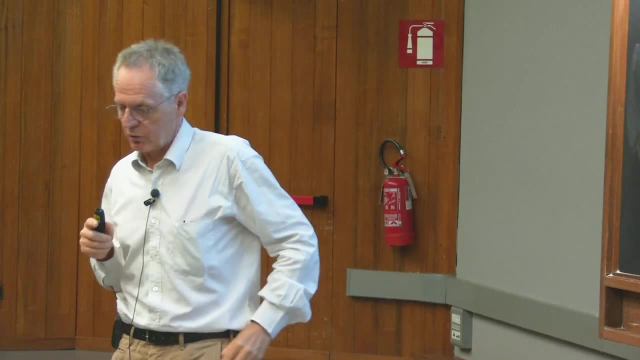 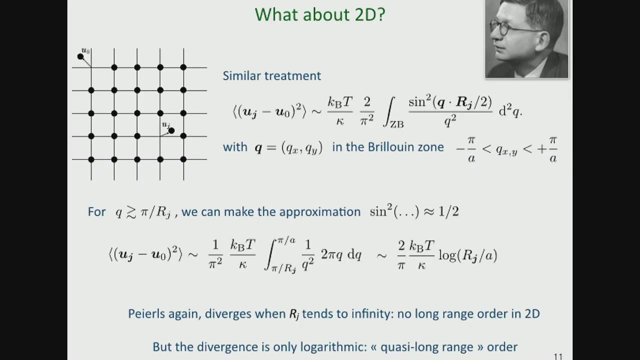 atoms are. if I look far enough, however, you see already a difference with respect to 1d. in 1d the divergence was linear rj. now it's only a logarithmic divergence, so it's not as strong as a divergence. so the loss of long range order. 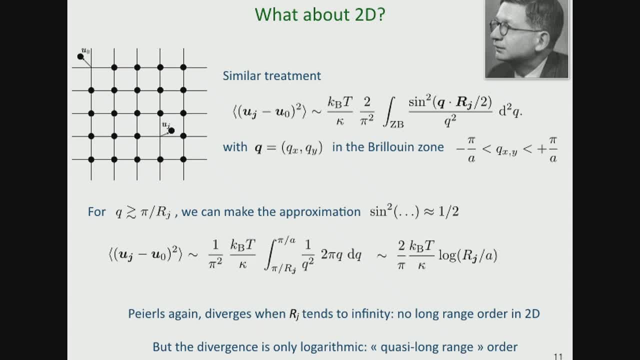 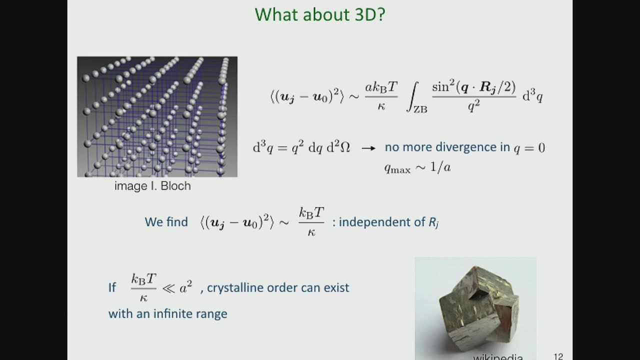 is not as big and people often speak because the divergence is only logarithmic, speak of quasi long range order instead of the total absence of long range order. and just to finish the argument, you may wonder what happens in 3d. so again in 3d you will have the same integral as: 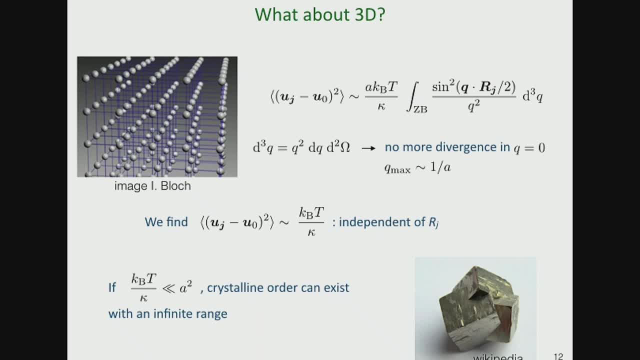 before. so you will get this kt temperature in front of the integral a sine square over q square. here now you will have a volume in momentum space, d3q, and when you replace this by polar coordinate, the d3q will become q square, dq, the q square. that will 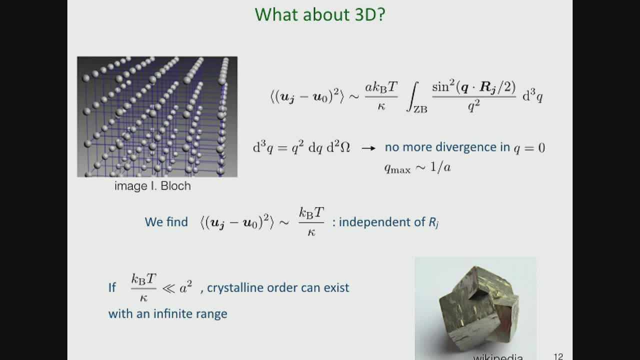 appear here, will cancel with this one. and now I have no divergence at all for low momentum. ok, so I had a linear divergence in 1d, I had a logarithmic divergence in 2d and now in 3d there is no divergence at all. so I can calculate. 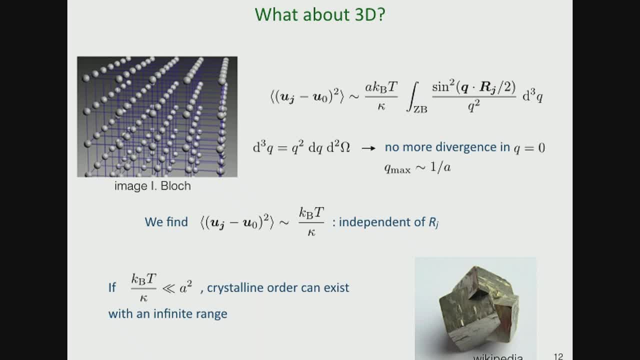 completely this integral and I get something which will be kbt over kappa, independent of rj, and this tells us that indeed, in 3d we can have true long range order if this quantity that I have here is much smaller than a square, which is again the square of the 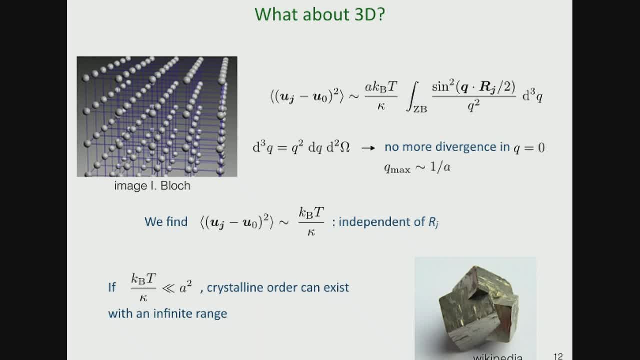 crystalline parameter, then if I know where an atom is sitting in this crystal, I will know where all the other atoms are sitting, within some fluctuations, which are given here, but these fluctuations are small compared to the lattice spacing. ok, and there is a criterion that this should be actually. 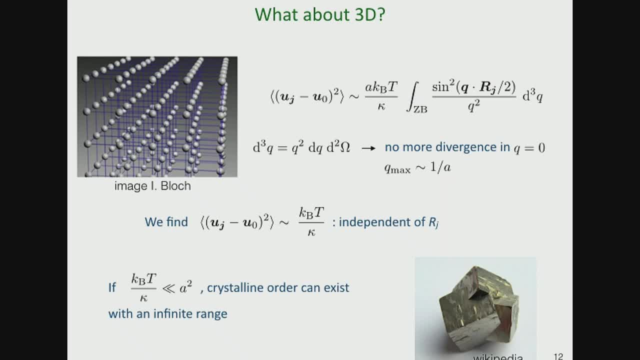 less than 10% of the lattice spacing if we don't want the crystal to start melting. so in 3d, with this argument I get true long range order, but in 1d and 2d I do not. and the physical reason for that? 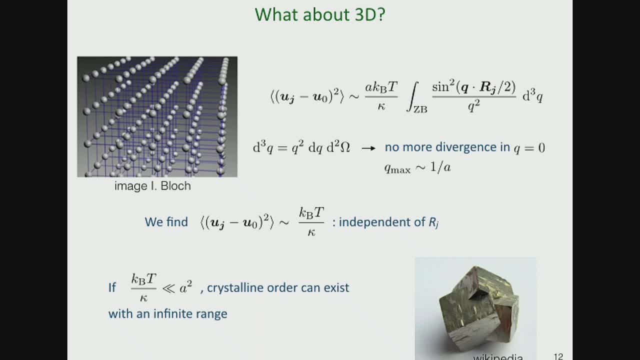 which is hidden in this math about Jacobian is the fact that when you are in 1d or 2d, you don't have enough neighbors. actually, when you are in 3d- and if I say that an atom wants to move out of its equilibrium position, it is going to. 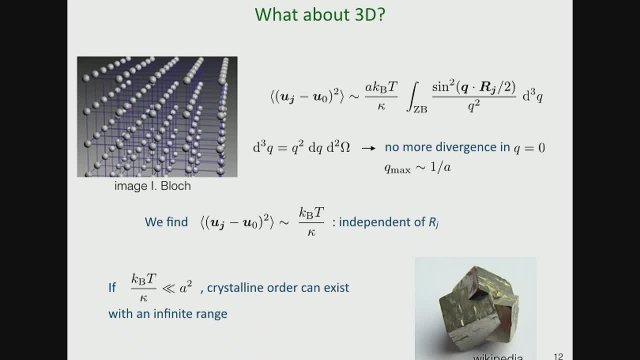 frustrate many, many people, people on the left and on the right, in front of me, behind me, people above and below, and so it is very unlikely that an atom can move a lot, because of there are many frustrations that are caused when the atom moves. when you are in 1d, you have only 2. 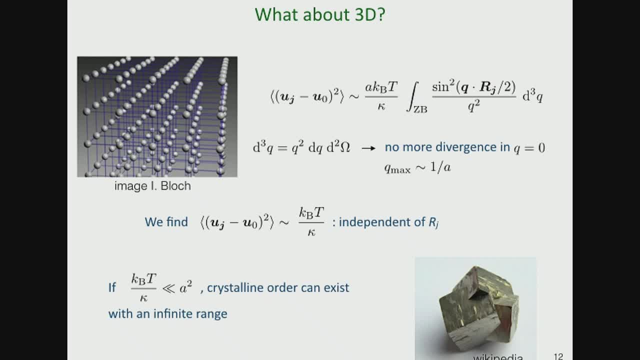 neighbors, one on the left and one on the right- and if you move like this, if this neighbor accepts to move also on the left, it is easy to have a big situation propagating and in 2d it is marginal and this is why we get a log. 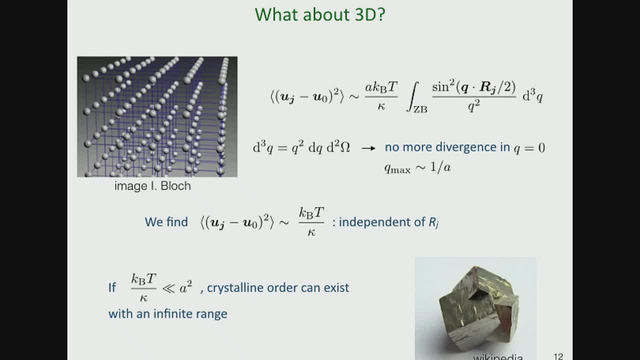 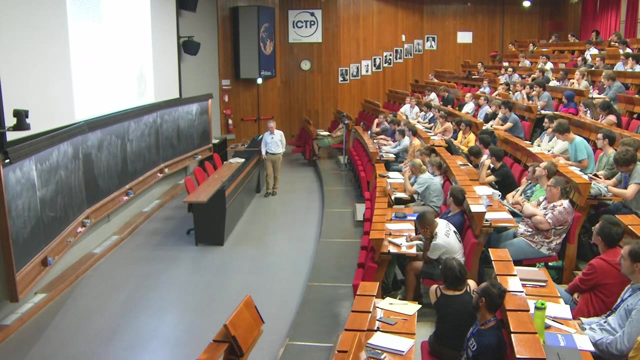 in 2d. okay, so the idea that I want to convey here is this lack of neighbors in low dimension which forbids to have true long range order. yes, ah, good question. yes, how does this apply to graphene? so there are two answers to that: in the literature and 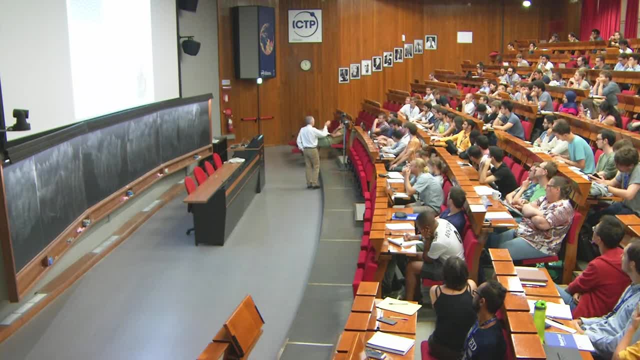 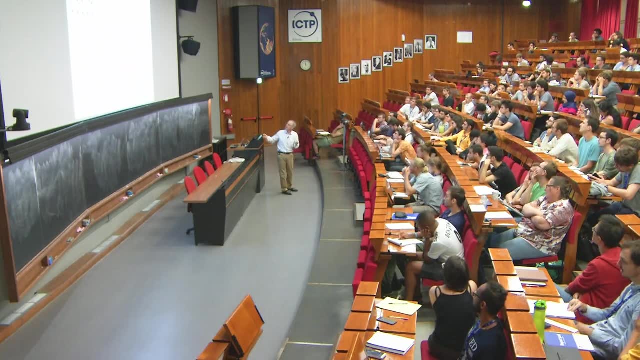 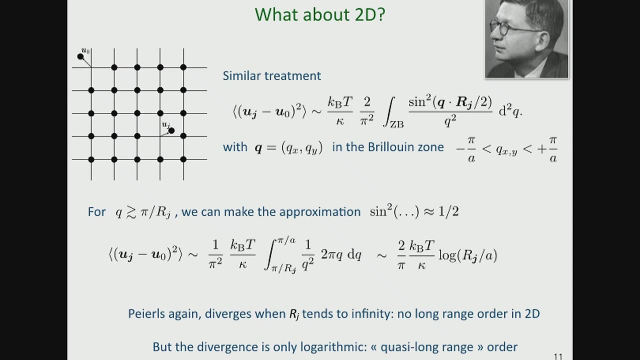 I don't think people have really, uh, completely say which one is correct. so one first reason is that when you took, when you take this in graphene and you take the value of kappa, the distance rj over which you lose the long range order is very, very long. 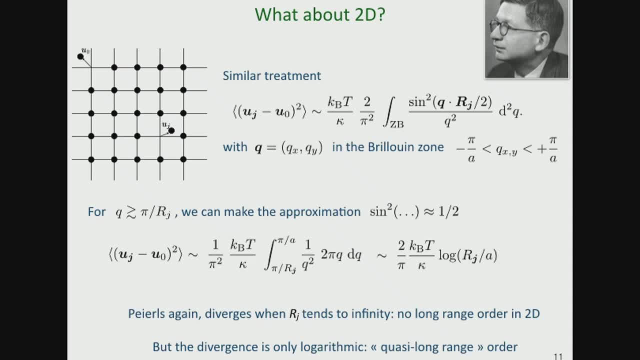 much larger than the graphene sheet that can be produced, so it's not so relevant for graphene from a practical point of view, taking into account the fact that the graphene sheets are micrometer size or tens of micrometer size. now there are some more elaborate arguments, which are 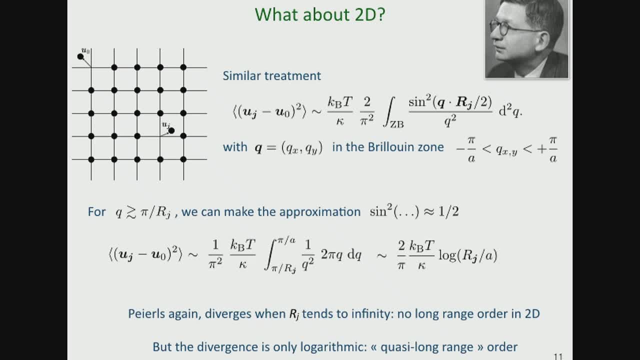 not actually, which could apply to even if we could produce infinite graphene sheet, which is that graphene is not really flat. graphene can bend and because of bending this introduce kind of long range interaction. that is, if I take into account the fact that the graphene sheet can bend like this. 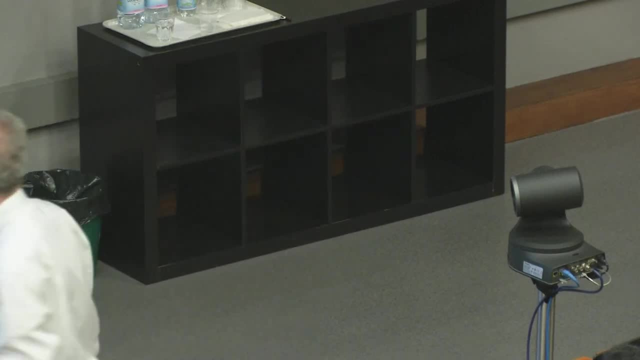 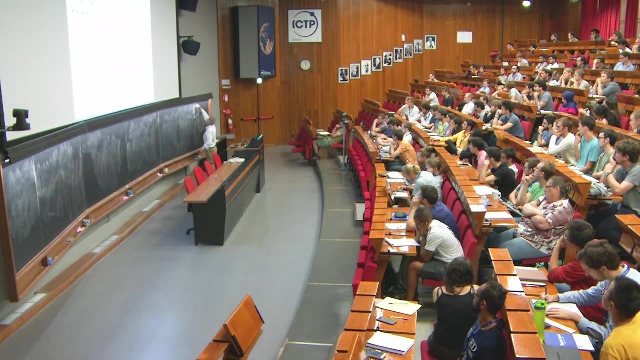 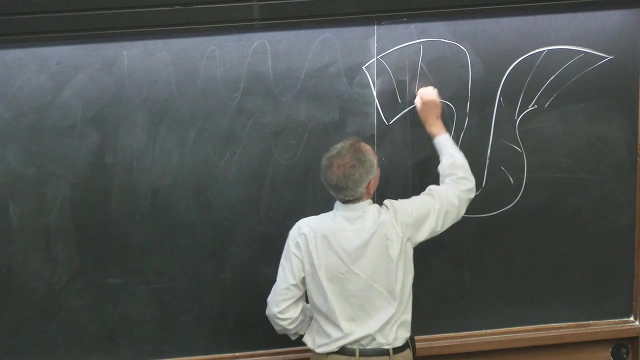 then I have interaction between two atoms. let me maybe draw my graphene sheet so you see what I mean. I'm not sure I can draw graphene sheet easily, but you see the graphene sheet that I'm trying to draw. yes, so I have an interaction between these two atoms when it bends. 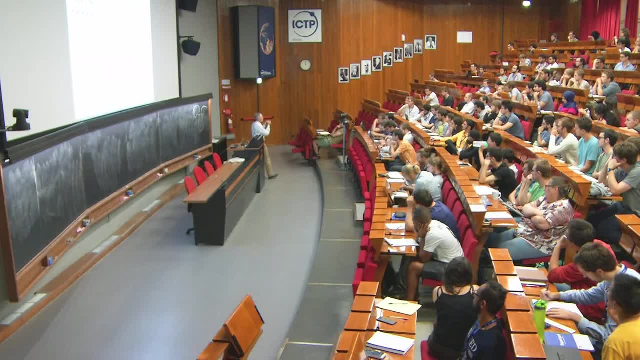 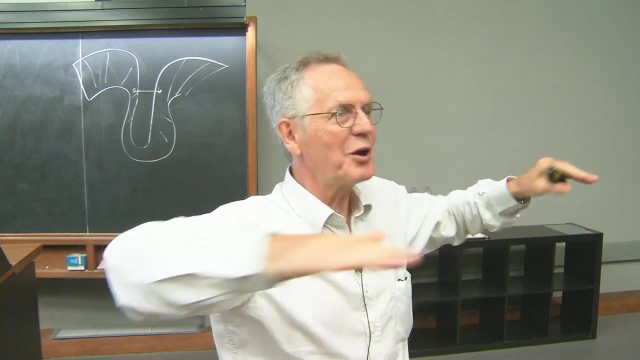 so this introduces a small component of long range interaction in the system because of the possibility of the graphene sheet to bend, and this is enough to restore, from a purely theoretical ground, the true long range order because of the bending. so graphene being not something which is flat but having 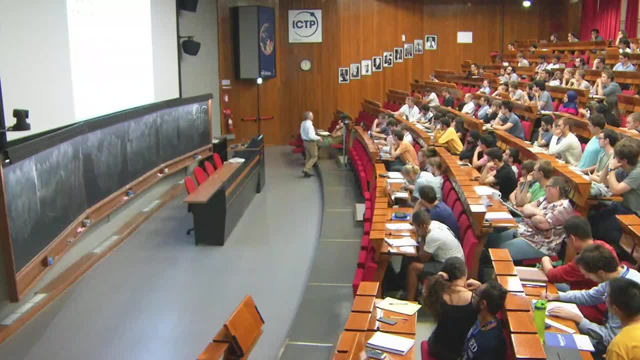 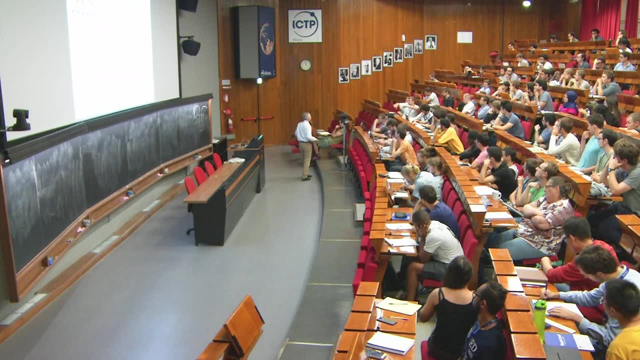 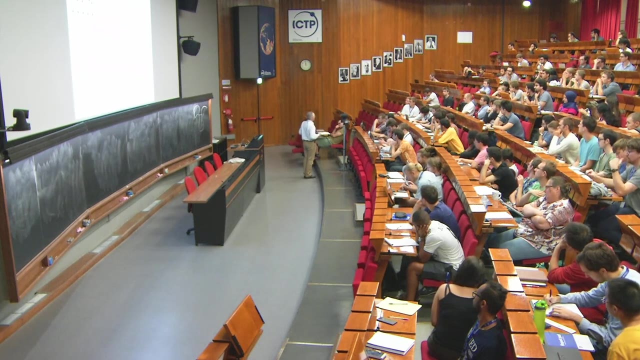 this possibility to bend. it's a cripple surface, if you want. yes, yes, so yes, a small bend is enough, because a log is very fragile, so it's easy to get rid of a log. if you introduce some new physics in the system, it's not solved and I'm not sure this is relevant. 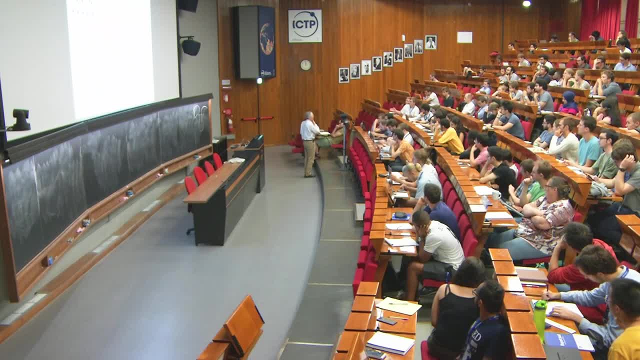 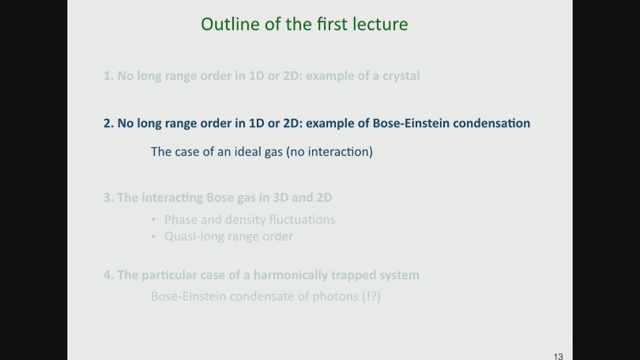 for any practical graphene sheet. ok, yes, then it might be relevant. yes, ok. so now that we have seen this example for the crystal, let's go to boson chain condensation, which is what we are interested in in this set of lectures, and first of all, I would like to start with the case of an ideal gas. 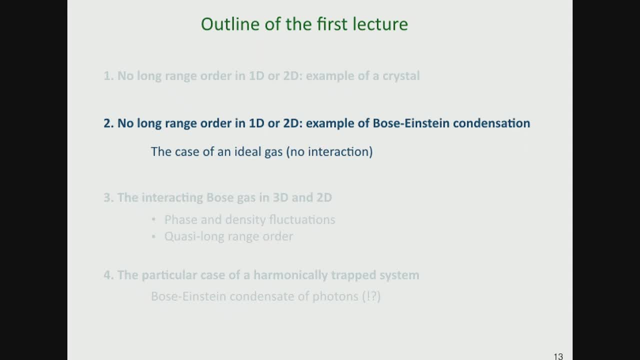 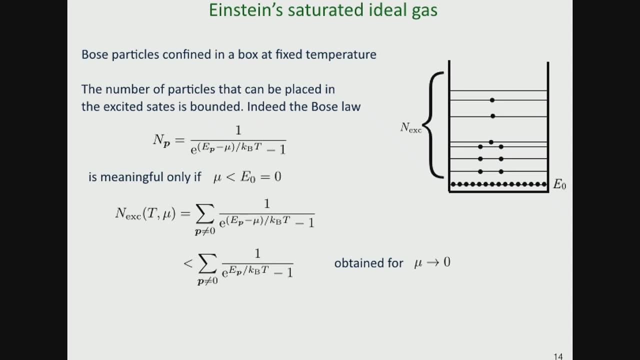 no interaction. so, again, these are probably some things that many of you have already seen. so I take particles, obeying Bose statistics, I confine them in a box at a non-zero temperature, and the first thing I would like to say is that, irrespective of the dimension, 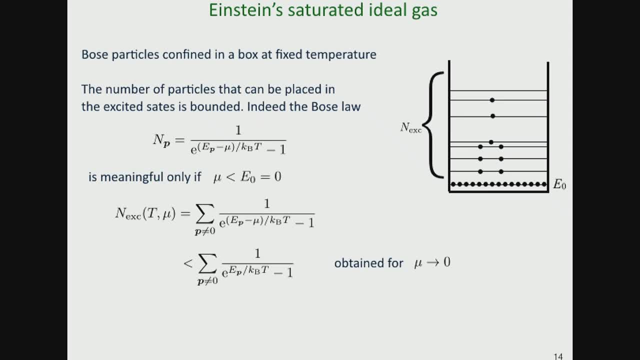 when I take a box or actually any kind of potential, I always get something that one can call boson chain condensation. that is, the number of particles that can be placed in the excited state of the box is always bounded, and indeed this comes from the Bose law. 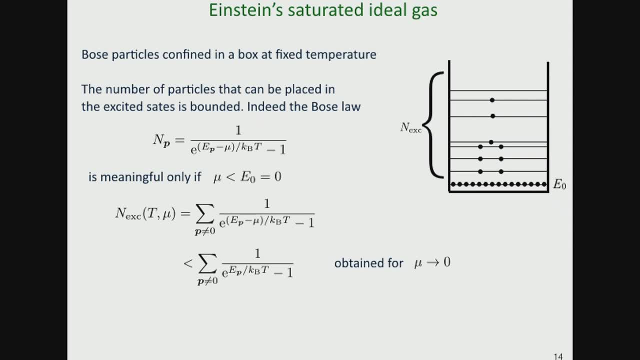 that I will use a lot, so I might as well write it on the board. so the number of particles on a state of energy E, as you know from the Bose-Einstein law, is the exponential of E minus mu divided by kB T minus one. ok, so this is something you have all seen. 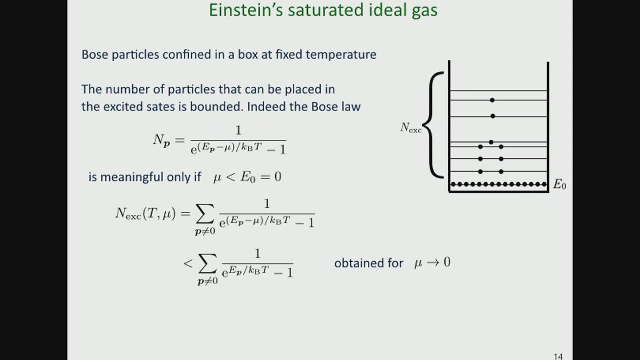 let's suppose that the lowest energy of the system is called zero, and I set it to zero, just a convention of energy. then in such a formula, the one which is written on the board mu has always to be smaller than E zero, which again is zero here. 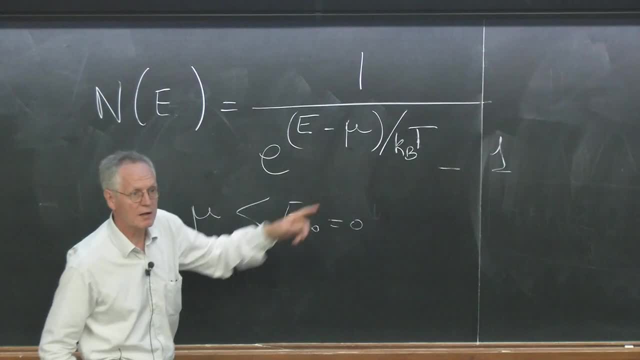 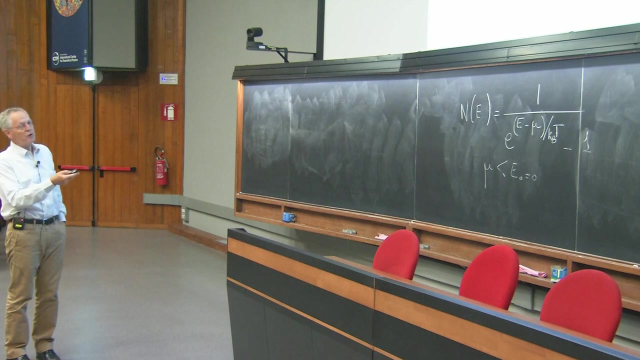 otherwise, if I allow myself to take mu larger than E zero, this will become negative and it will be nonsense. so in a Bose-Einstein system, by contrast to Fermi system, the chemical potential is bounded lower than the energy of the ground state and therefore just a mathematical exercise. 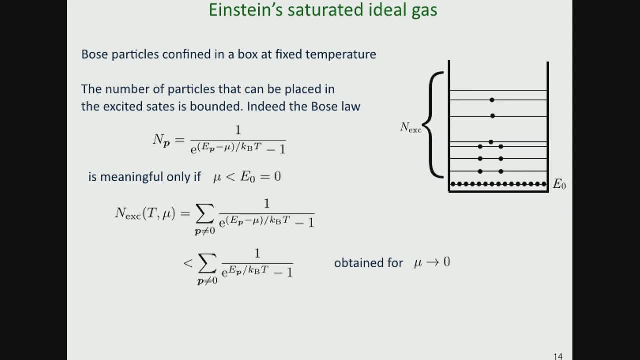 to see that if I take the sum of all, of all the population, but the ground state here, so I exclude p equals zero from this- from this sum, this sum here is always smaller than the same sum without the mu here. and this quantity, if I take a discrete sum, 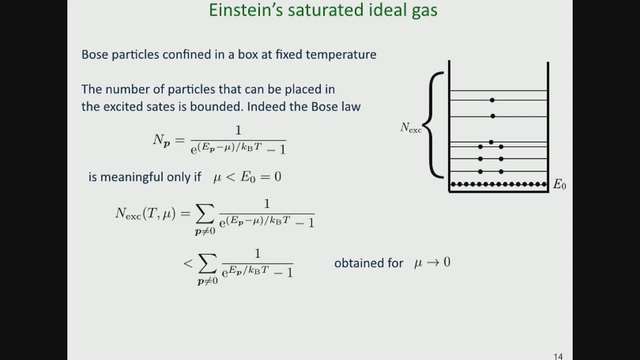 I can calculate it and therefore the number of particles I can put in the excited state for this temperature and this chemical potential. mu is always bounded, which means that if I take the same temperature and I constantly add particles, that mu is going to vary because mu is always smaller. 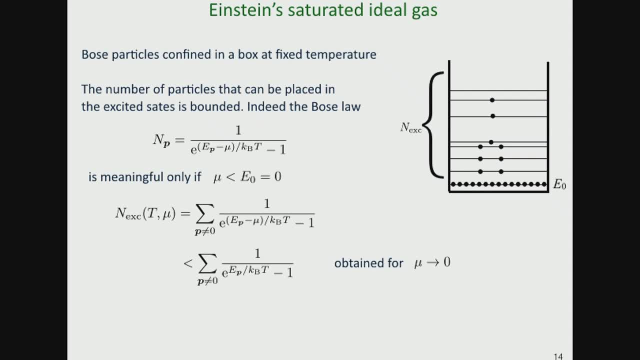 than that the number of particles in all the excited state. so in this sense, Bose-Einstein condensation in a finite system with a discrete level is very simple. just an inequality like that and you don't have to discuss anything more. and this will be true in 1D, 2D or 3D. 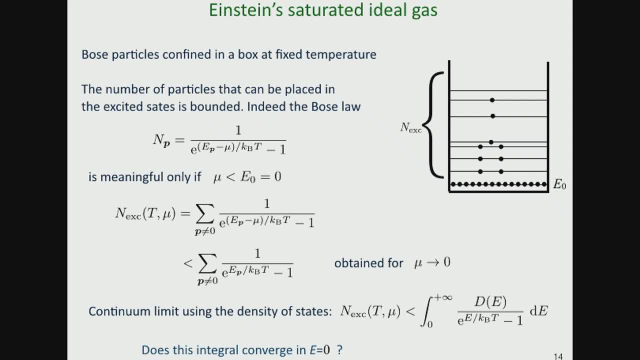 now the question that was not trivial in Einstein's paper and which has actually caused a lot of debates, is that the size of the box tends to infinity. if I keep constant the temperature and I let the size of the box tend to infinity, keeping the same density, 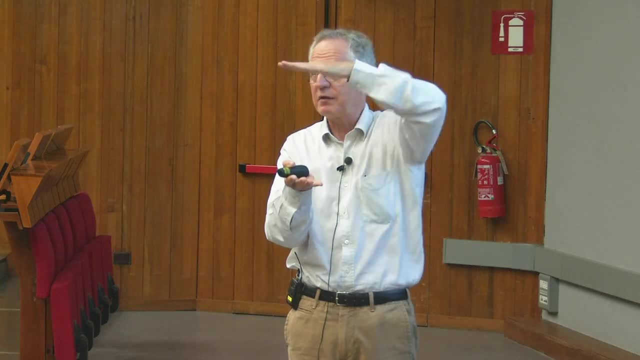 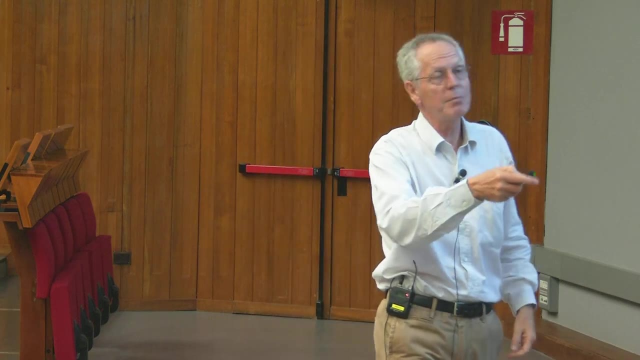 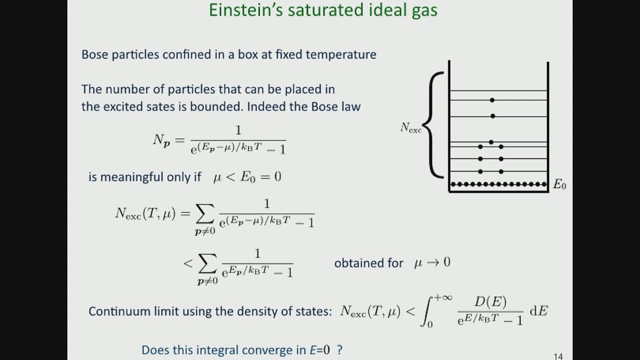 then what happens? and when you do that, the discrete structure of the level will disappear. I will transform my discrete set of states into a continuum. so I have to go to replace the expansion of E over kT minus 1, and all the question is again related to low wave vector. 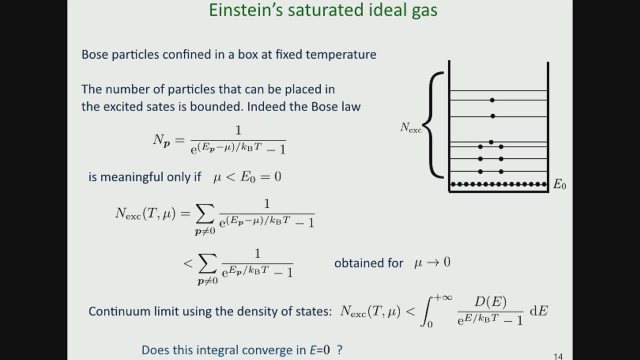 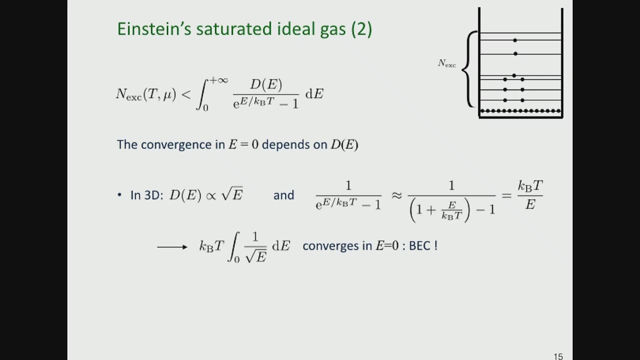 low momenta or, if you prefer, low energy. all the question is: does this integral converge? and does it converge in E equal 0 and, as you probably all have seen, it depends on the shape of this density of states. so, if you go so, I have rewritten this integral here. 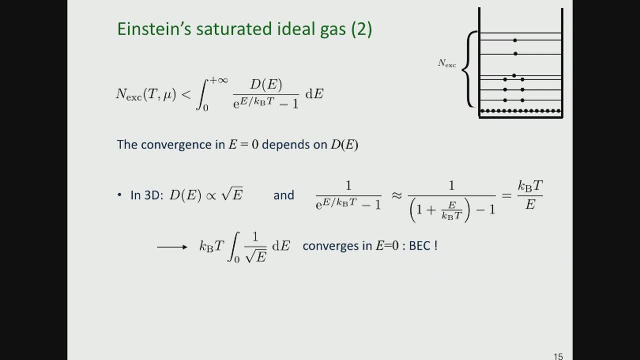 if you go in 3D, the density of state in a cubic box tends to infinity, varies like the square root of the energy, and the denominator here for low energy is typically linear in energy. so you get an integral which is square root of E divided by E. 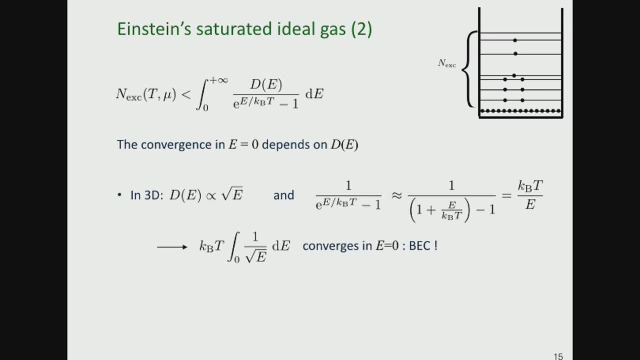 so 1 over square root of E and this integral converges in 0 and therefore the number of states you can put in the excited states remains bounded when you take the number of particles, or more precisely the density when you take the thermodynamic limit, remains bounded. 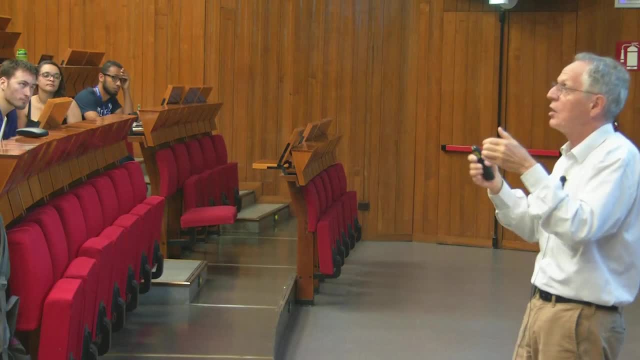 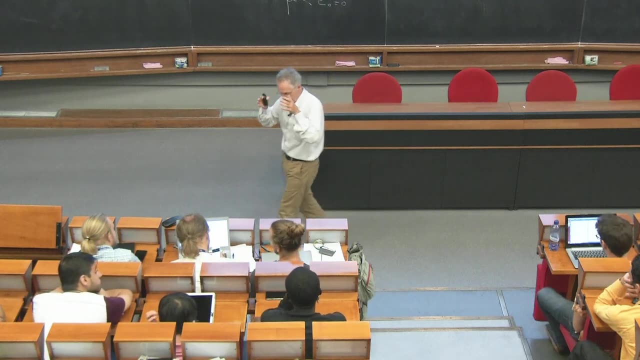 and therefore this Bose-Einstein condensation that we had for finite size system survives when you take the thermodynamic limit because this integral converges. so again for a discrete system, you always have BEC and when you take the thermodynamic limit, if this integral converges. 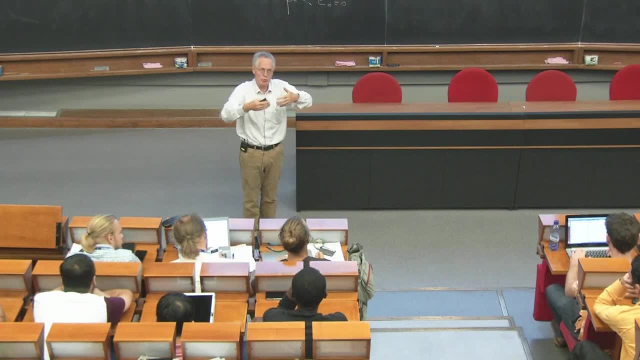 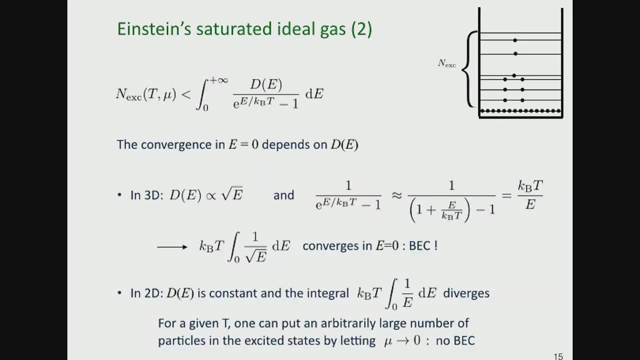 it means that the density that you can put in the excited state is bounded and therefore you will survive, and this is the case when you go to 2D. the density of state d of E is constant and therefore the integral that you have to calculate now is 1 over E. 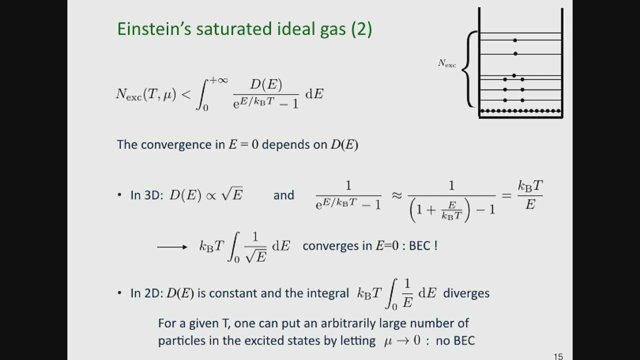 because the denominator is partial to E and this integral diverges, which tells you that the Bose-Einstein condensation phenomenon does not survive. when you take the thermodynamic limit, the density that you can put in the excited state now can be infinite and therefore there is no macroscopic accumulation. 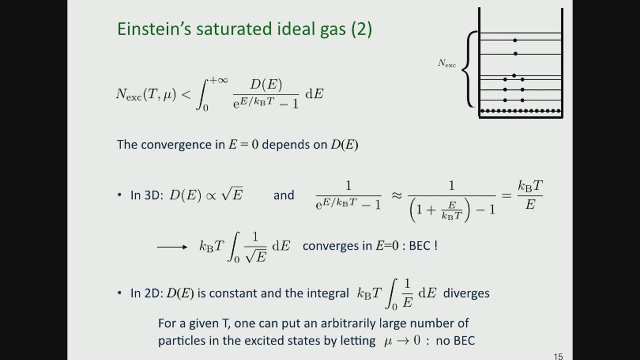 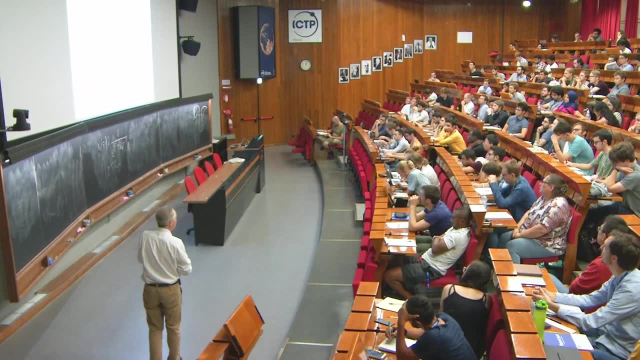 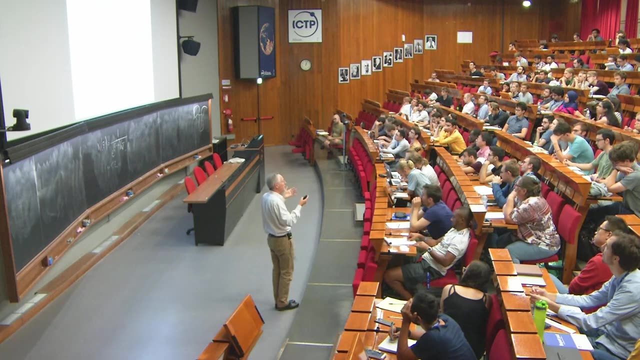 of particles in the ground state. I wanted to make this clear for everyone. is it ok? no question, ok. so still, it is interesting to see what happens when you take a Bose gas in the thermodynamic limit in two dimensions and see where do the particles go. 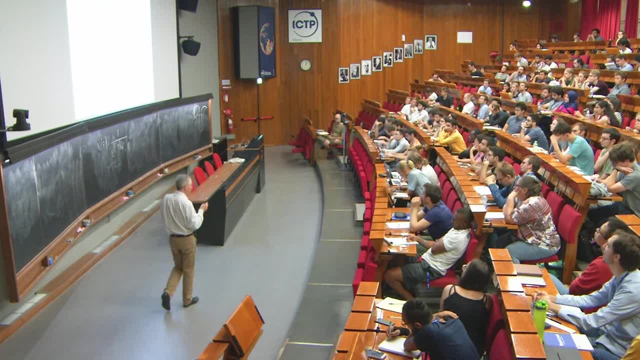 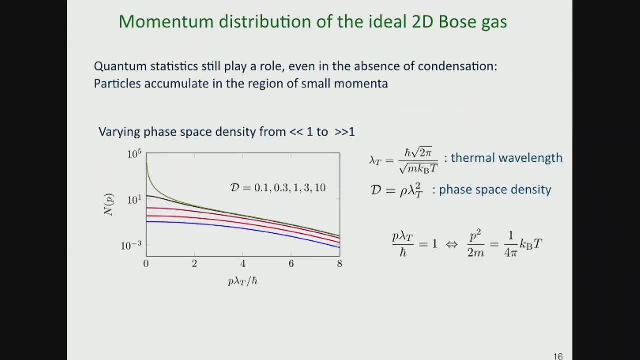 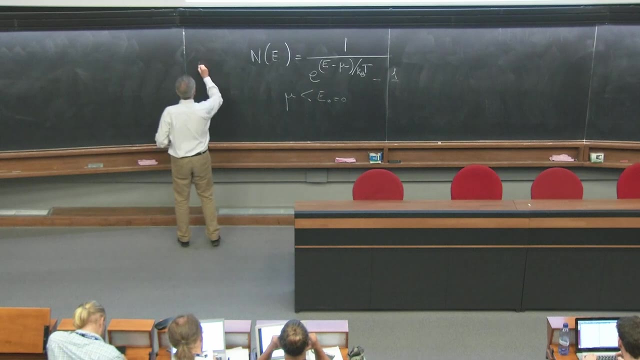 I told you that they do not accumulate in the ground state, but still there is a kind of saturation which occurs. and in order to show that I have taken this Bose-Einstein law, which is written here, so I take: I am in a box, so I take E equal p square over m. 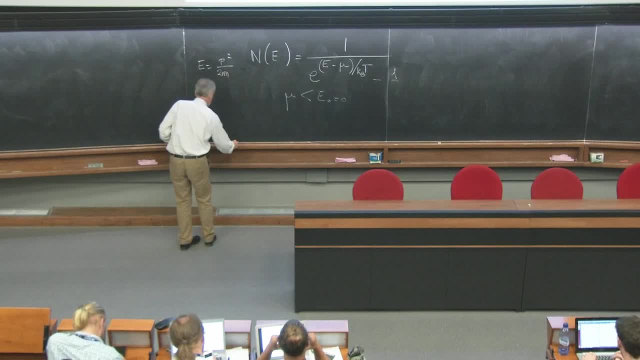 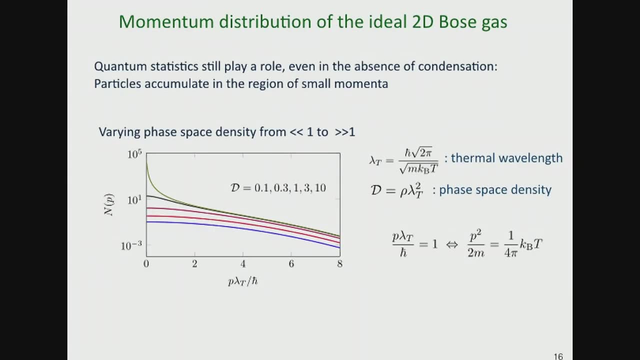 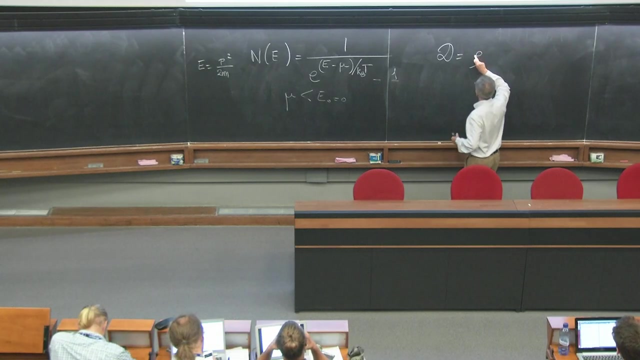 over 2m and I plot here the density distribution in this box for various phase space density: rho times, lambda square. so this is the quantity that I will use a lot. so the phase space density d is the density. special density: rho times, lambda square. lambda t square. 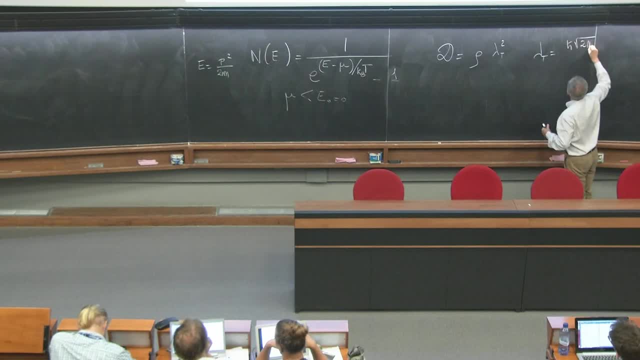 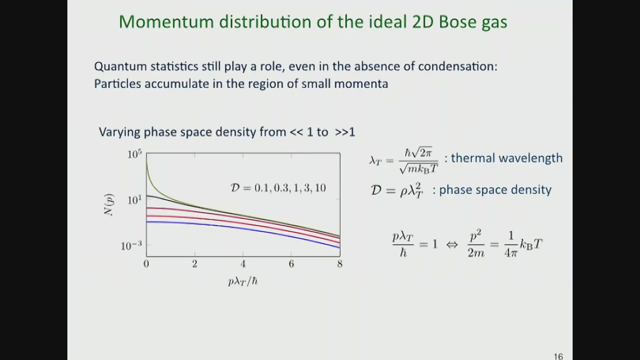 is equal- I just rewrite it here- square root of m, k, B, T. so varying the phase space density is a way to vary the degeneracy of the gas go from the classical regime to more quantum regime. so here I have plotted in various colors the momentum distribution. 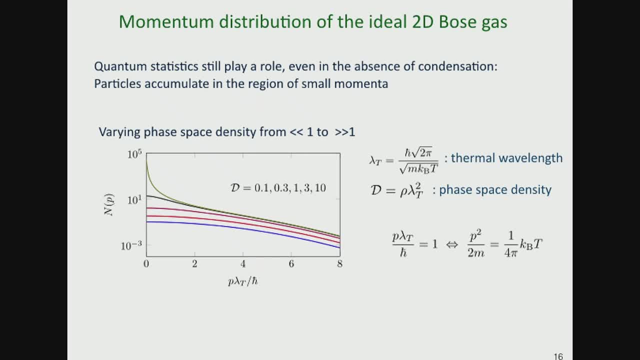 n of p in the box as a function of momentum p for various phase space, density of 0.1, so gas which is very weakly degenerate, kind of Maxwell-Boltzmann gas. so n of p is just a Maxwell distribution, a Gaussian distribution. 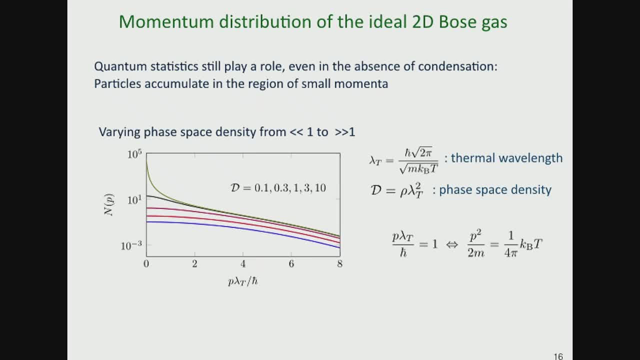 here I have taken some logarithmic coordinate here, so a Gaussian with a logarithmic, semi logarithmic coordinates correspond to a parabola like that, and this is a blue curve, the unit that I put here, so it's the momentum, p, dimensionless variable. so I use p lambda, t over h bar. 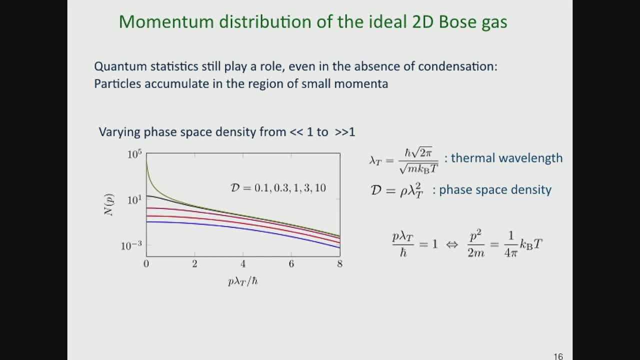 when this is equal to 1. if you square it and you replace you take the value of lambda t which is written on the board. here you get p square over 2 m, equal 1 over 4, pi, k, B, T. so this corresponds to the situation 1 here. 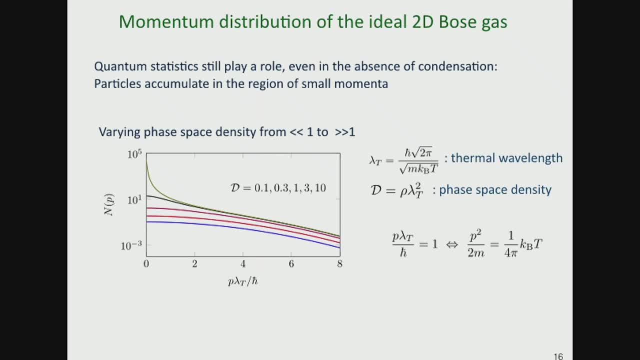 is when the kinetic energy is on the order of k, B, T, so at low phase space density. no surprise, this is Maxwell-Boltzmann. when I increase the phase space density, I am accumulating in low momenta, momenta which are such that p lambda, t over h bar. 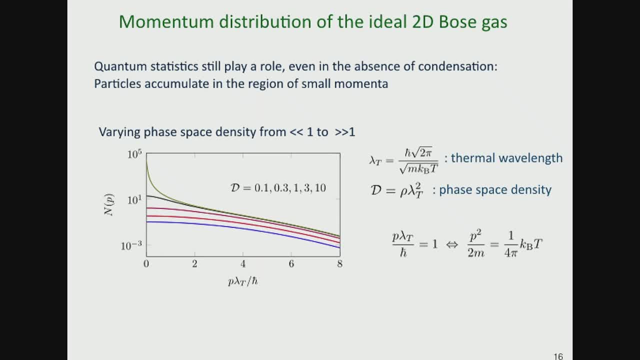 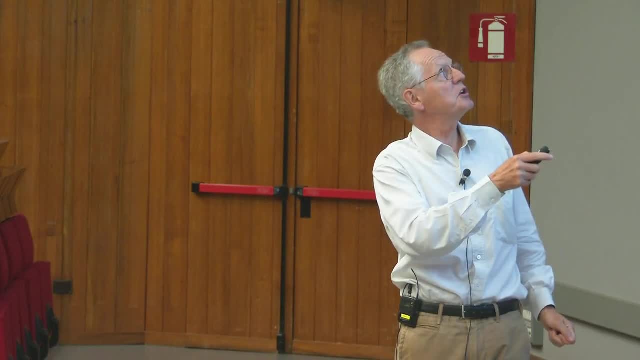 is smaller than 1 or, if you prefer, the kinetic energy is smaller than k, B, T. so you see that more and more. when I put more and more particles I don't get a Bose-Einstein condensate. because I am in 2D, a Bose-Einstein condensate would be. 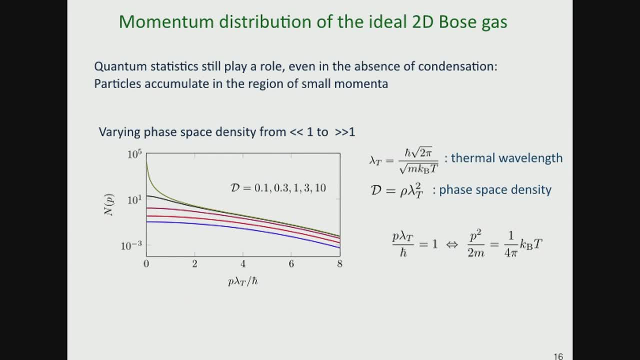 an accumulation of particles in p equal 0, which is not what I see. but I see that the particles accumulate at low momenta here. the high momenta here are nearly saturated. at large momenta all the particles go to low momenta but not to a single one, like in 3D. 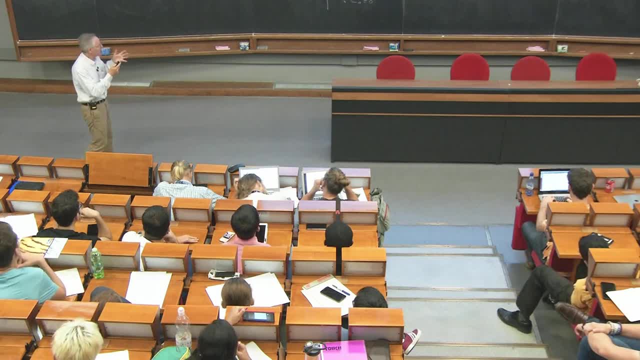 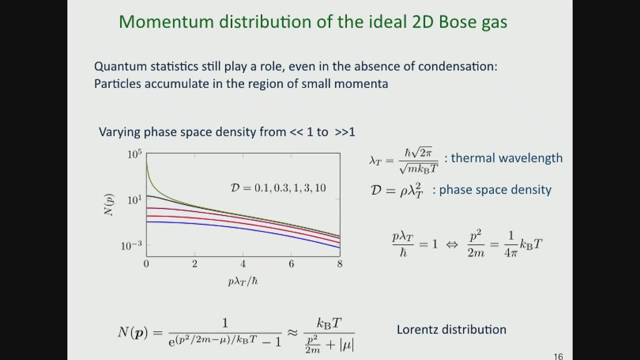 but to a continuum of low momenta, which is here and this is what happens for this ideal gas. and if I look at what happens at phase space, density of 10- actually this is not obvious because I am using logarithmic coordinate, but most of the particles are now. 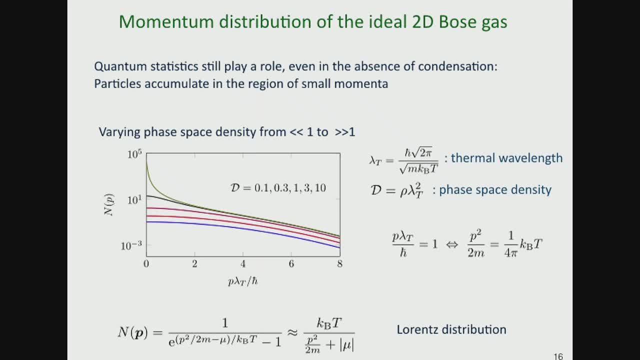 sitting in this low energy tail here and very few particles are here by contrast. and if I now ask myself what is the shape of this momentum distribution close to p equal 0, then I can take again this equation here and I say that e minus mu over kt. 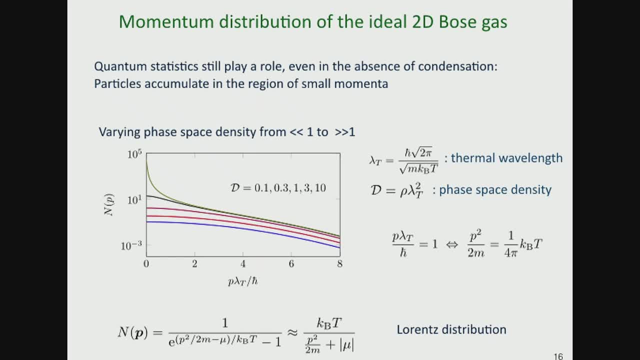 is a small variable, so I can expand the exponential and I get now that this n of p, when I expand, will be kbt divided by p square over 2m plus mu, which is a Lorentz distribution. so in 2D when you cool a gas. 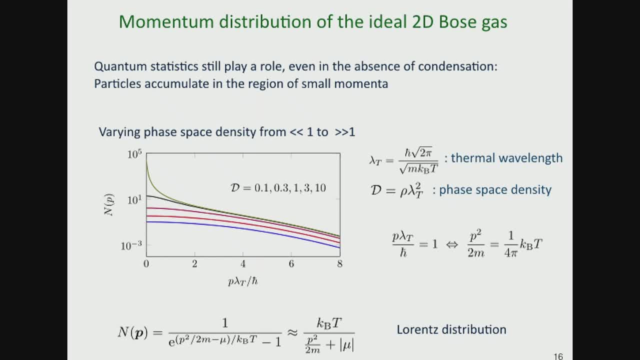 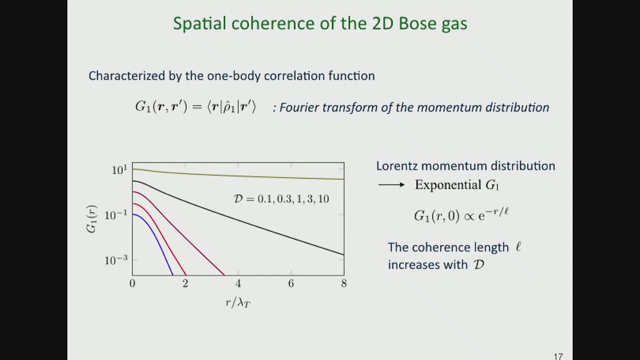 a Bose gas. what you get is that most of the particles are strongly degenerative. most of the particles accumulate in the low momentum class and they have a momentum distribution which is a Lorentz distribution like this. so now you may ask: what does it mean? with respect, 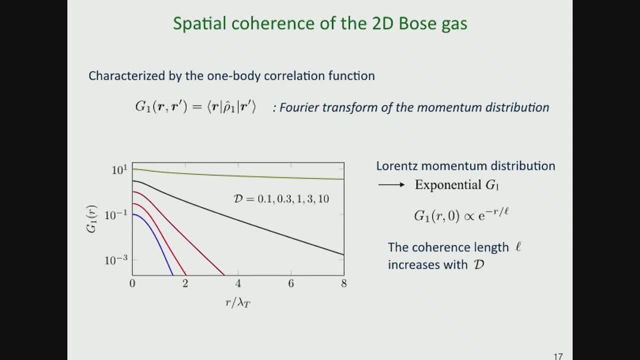 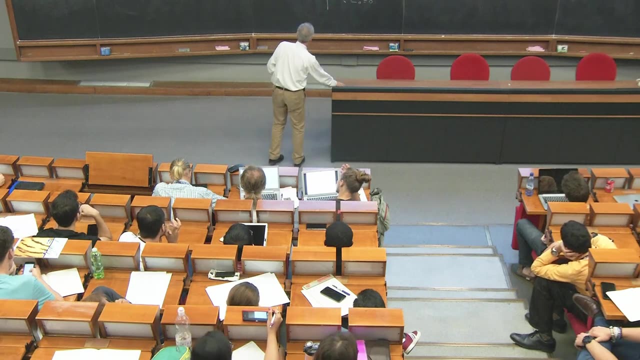 to the absence of long range order, and the long range order in a Bose gas is characterized by a quantity I introduced in the colloquium yesterday. this is a g1 function. this is how the phase is correlated between one point in r, so the definition I had yesterday. 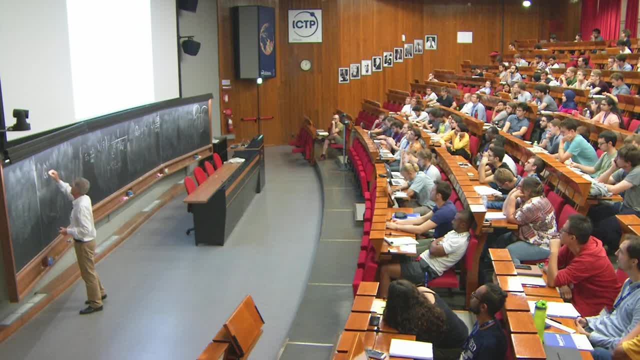 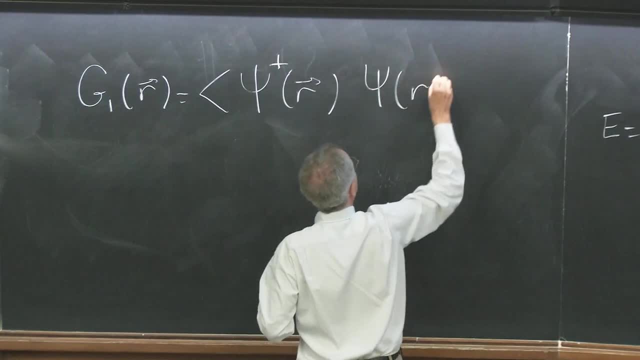 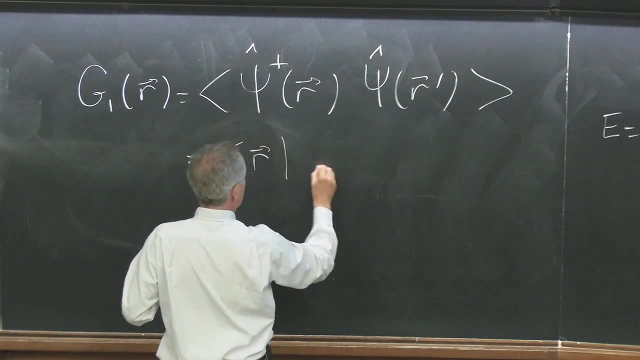 was. two definitions are equivalent, so g1 of r. yesterday I think I wrote that it was psi dagger of r, psi of r prime, where psi is the field operator, but this can also be written. it's equivalent to r. so one body density matrix: rho1 r prime. 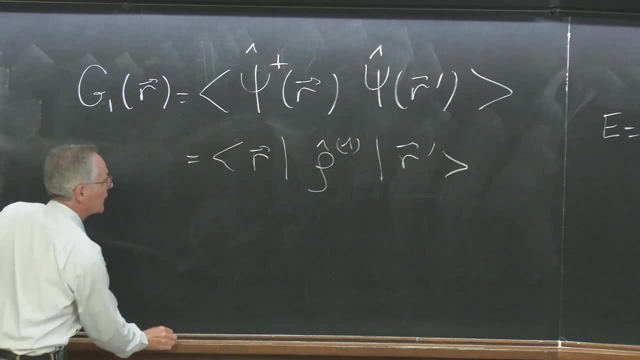 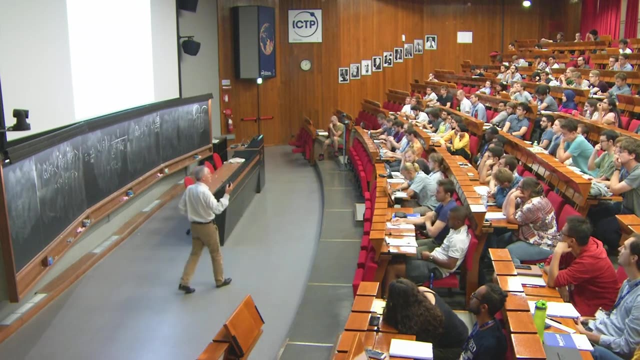 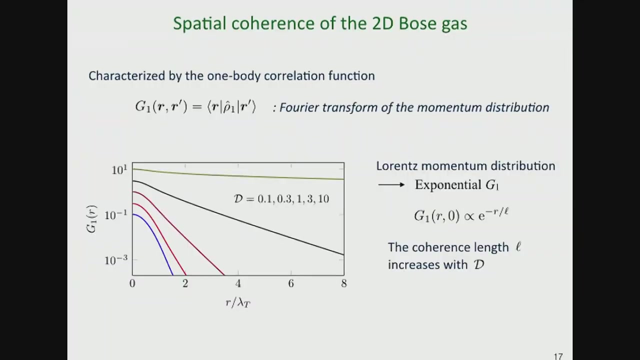 these two definitions are equivalent. this can be shown easily, and so because this one body correlation function- I can let you show this as an exercise, it's relatively easy to show- can always be calculated from the momentum distribution, because these two quantities are just rated by a Fourier transform. 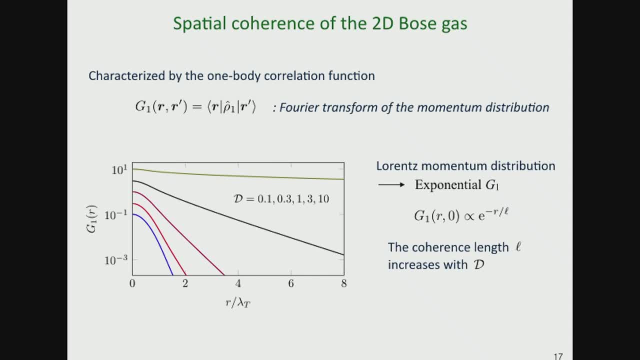 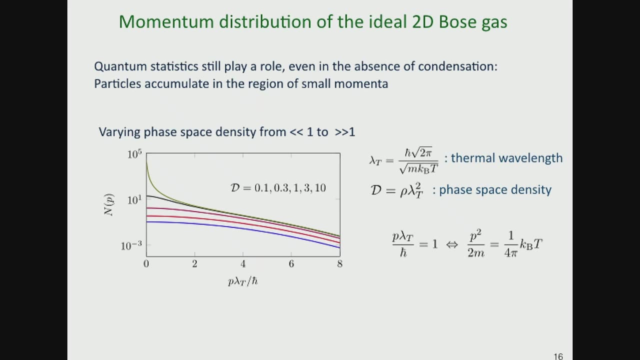 that is, if you want to calculate g1 of r, you can take the momentum distribution n of p, and n of p is the Fourier transform of g1 of r, and vice versa. so now we know that the momentum distribution is: this is what was here, is a Lorentzian, at least. 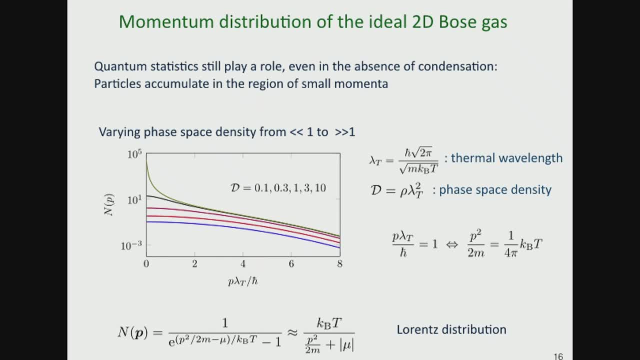 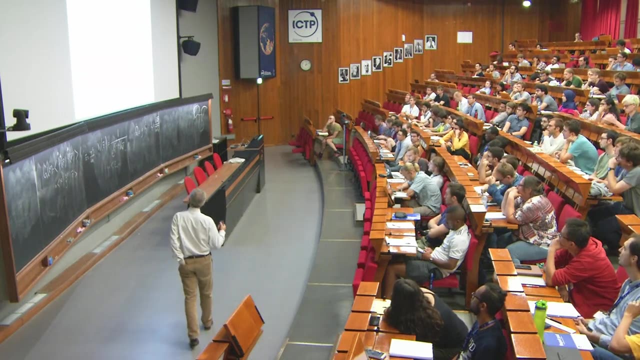 at low momenta. so we have to know what is a Fourier transform of a Lorentzian? and the answer is: do you know what? it is an exponential. exponential minus r over l, and so what we get for this ideal Bose gas, is that indeed? 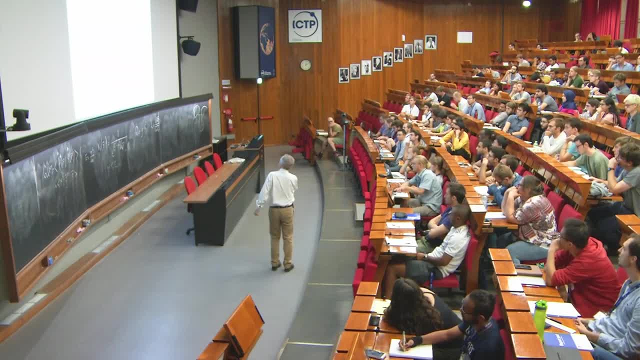 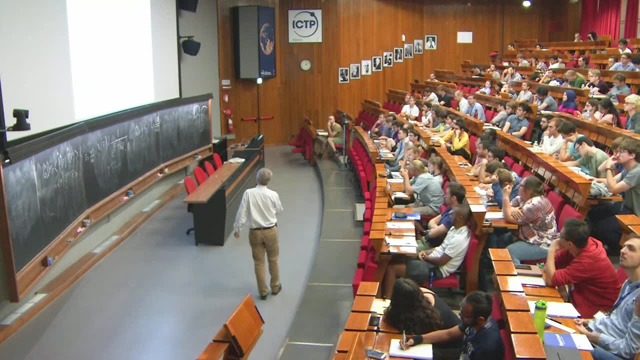 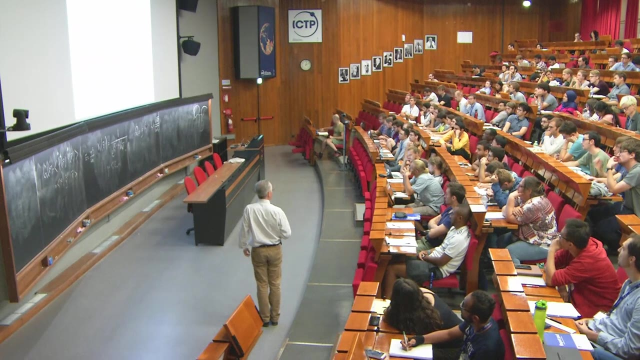 Peierls again is correct. there is no long range order. so the momentum distribution decays exponentially with the distance between the two points I am considering and with the length l, which increases when I increase the phase space density, but still it always decreases exponentially, exponentially fast. 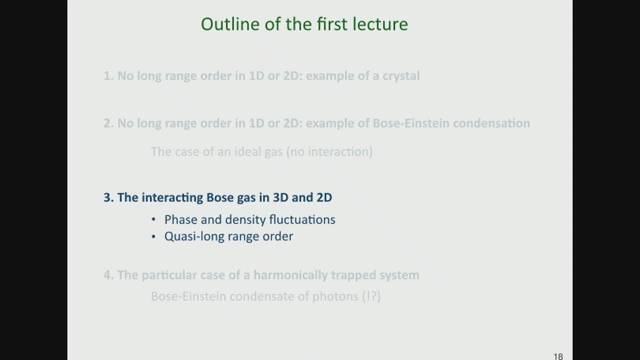 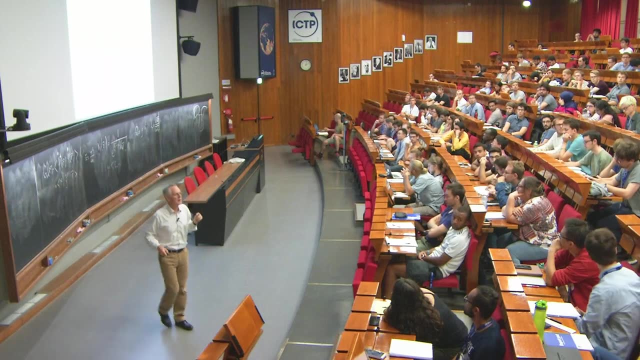 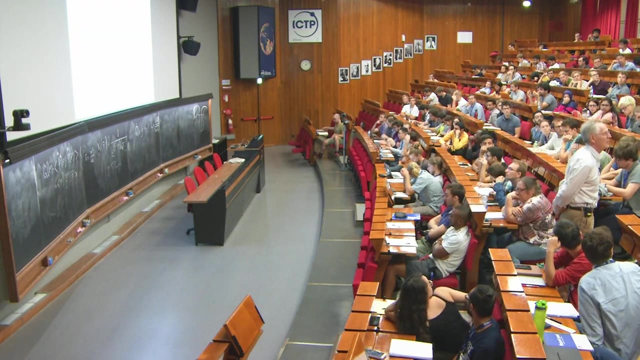 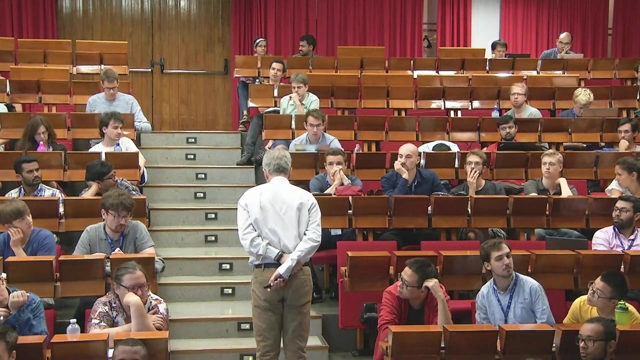 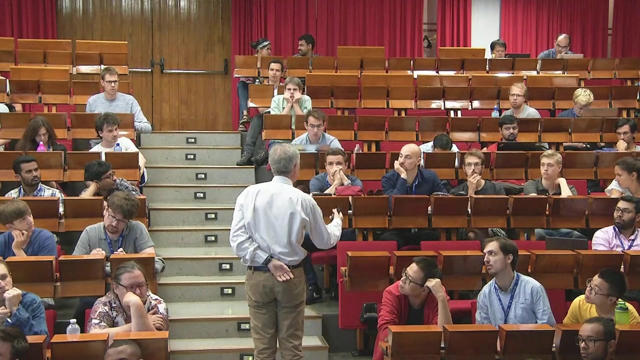 ok, so how am I doing in time? yes, I still have something like 15 minutes, so are there questions at this stage? yes, yes, yes, yes, yes, yes, yes. so the question is: do you need a Bose Einstein condensation to get ITC superconductivity or to get superfluidity? 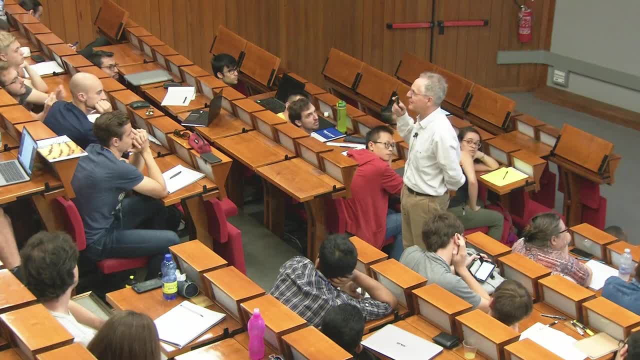 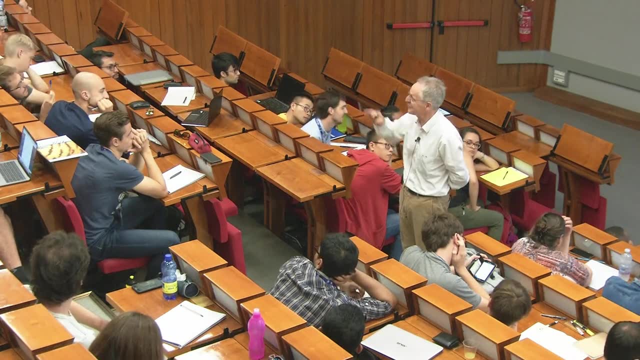 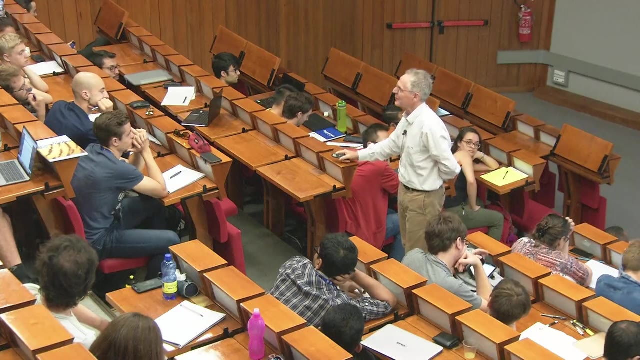 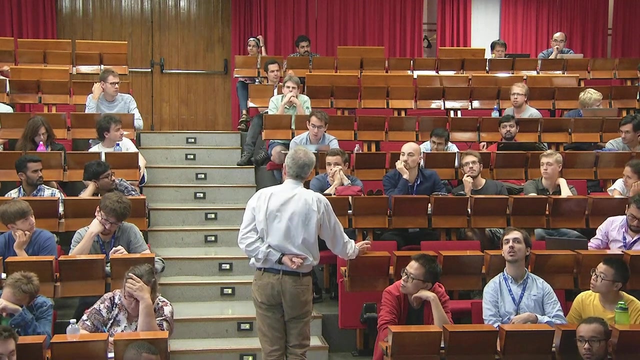 and the answer is no, you can get. this is precisely the work of. you can get superfluidity without yes, no, no, you should not be sorry. this is a very important point. thanks for pointing it. ok, so probably what Emmanuel had in mind was a quasi condensation. 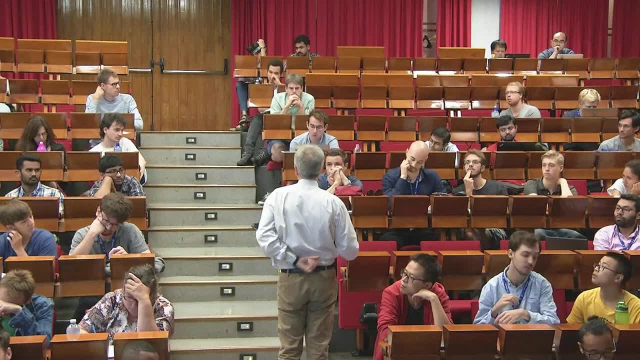 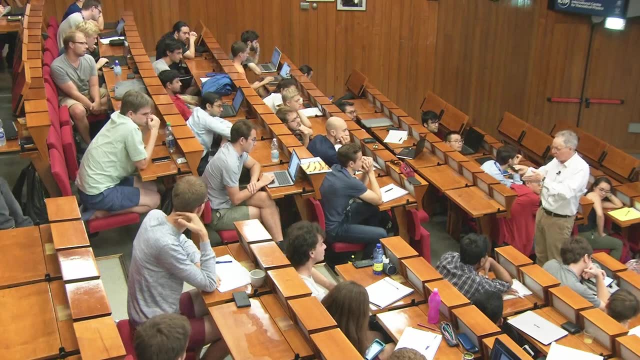 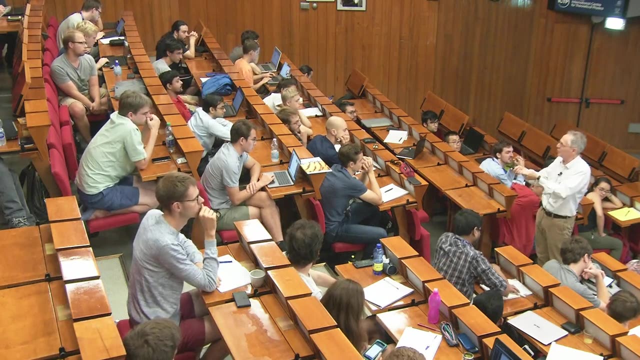 so quasi long range order, which was enough to ensure everything he was saying. so this was the answer for the graphene sheet. if you are looking on a short distance where the log has not time to rise, then everything happens as if you had long range order because you are looking between points. 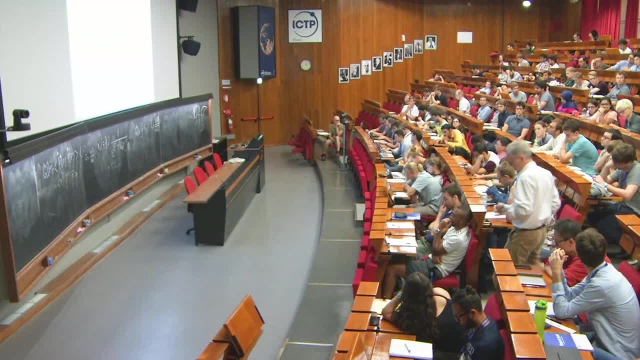 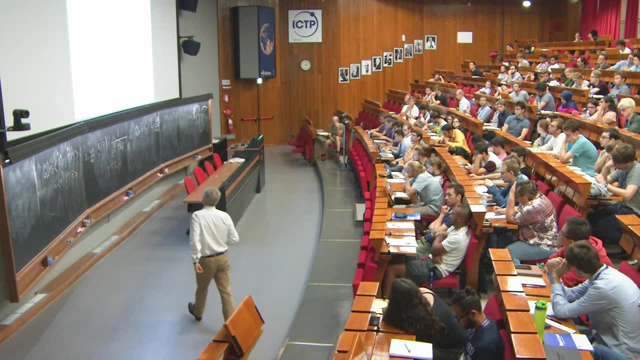 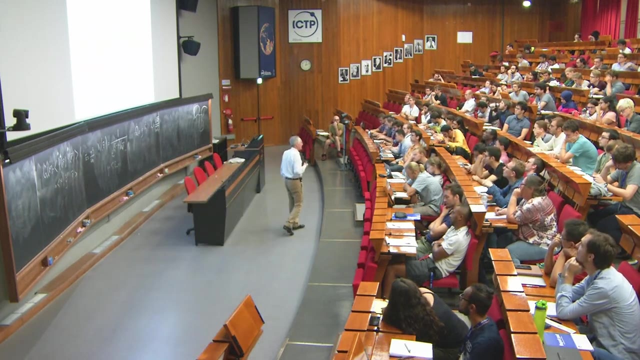 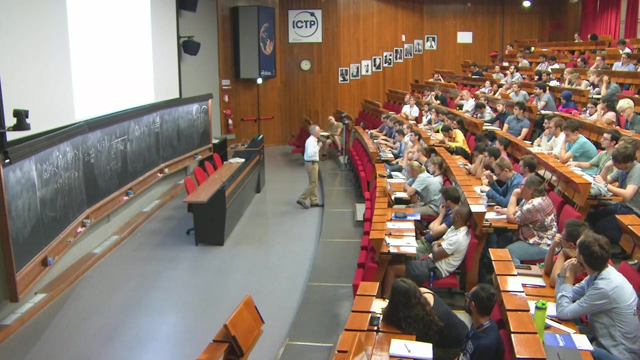 which are relatively close to each other. ok, other questions? no, let me now go to the case of an interacting Bose gas, which is more interesting but also more challenging, and you will see that interactions still do not violate Mermin-Wagner theorem, but still they change a little bit. 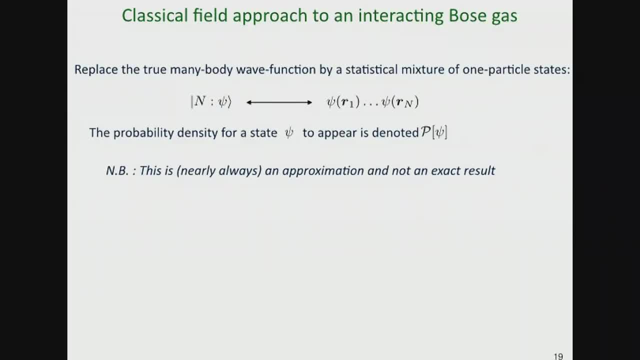 the picture that we have for the ideal gas of this exponentially decreasing G1 function. so in order to discuss the interacting Bose gas one has to do some approximation and you can never treat exactly an interacting many body system, at least in two dimensions or three dimensions, and the approximation 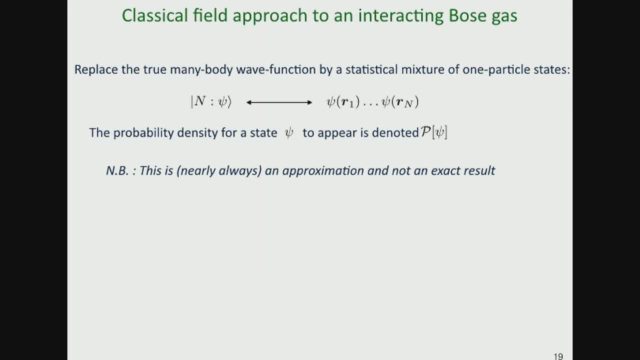 I am going to use is a so called classical field approach. that is, this classical field approach amounts to say that we have a true many body wave function, which is a complicated object, but we are going to replace it by an ansatz which is often called the Hartree ansatz. 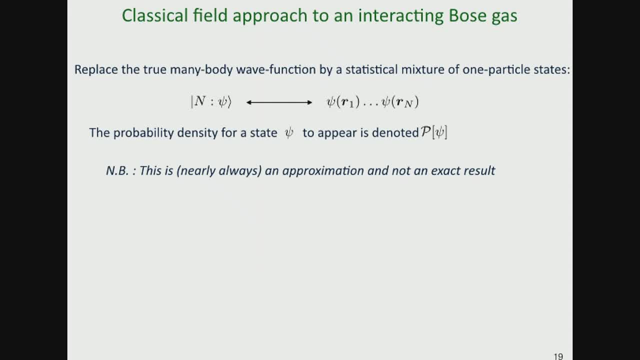 which is to say that all particles occupy the same state, psi. so I write this either as n psi, like this, or, if you prefer, r1 inside psi, r1, particle 2, psi, r2, particle n, psi, rn. but the psi itself is a fluctuating object. 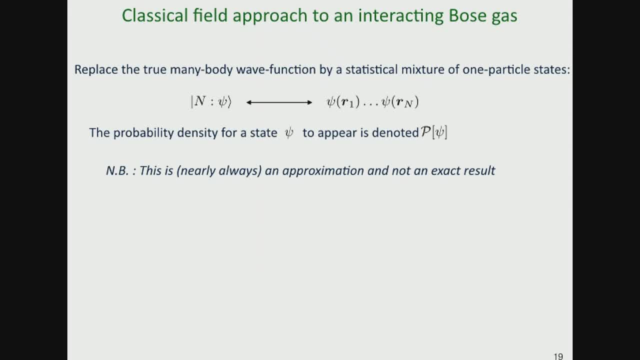 if psi was the ground state of the box, this would be a Bose-Einstein condensate. but here I take for this psi a fluctuating object, a fluctuating field, but I assume that all the particles are occupying this field, so it is not an exact result. 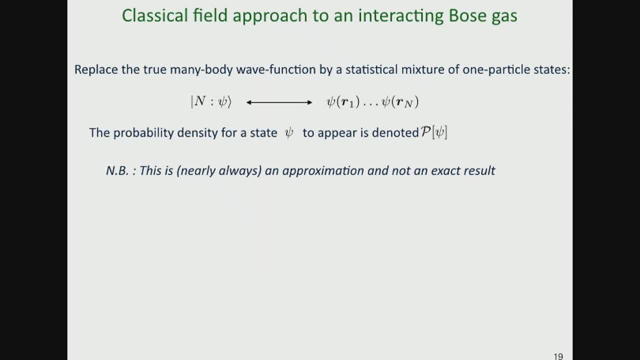 but it is an approximation and the rule of the game is to find the distribution for this classical field, psi. so this may sound a bit strange as an approximation, but for those of you who are familiar with electromagnetism, this is exactly what you do when you do classical electromagnetism. 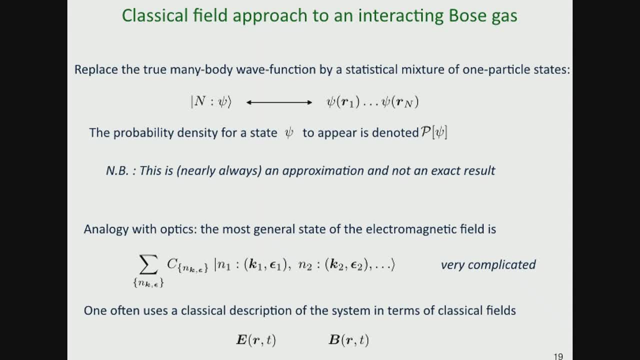 if you want to describe a field using quantum electrodynamics, you have to use some very complicated state where you have to specify the number of photons with momentum, k1, and polarization: epsilon1, k2, epsilon2. this is very hard to manipulate, but we all have learned classical electromagnetism. 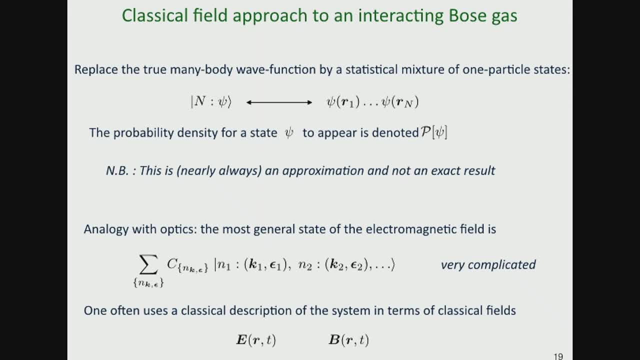 where we describe our electromagnetic field by a classical field, actually two classical fields: the electric field and the magnetic field. so when you are doing classical electromagnetism, you are doing exactly what I am doing here. here you are saying that all the photons, so to speak, share the same wave function. 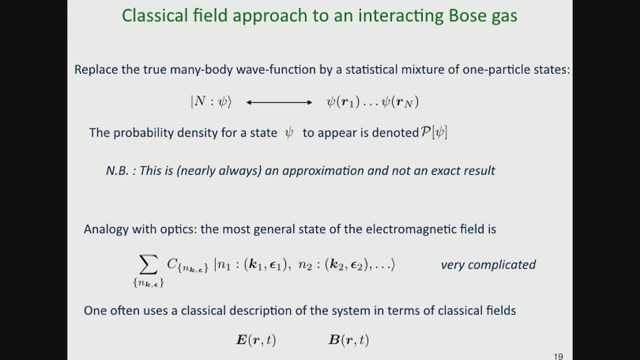 it is always dangerous to speak of the wave function of a photon- but are described by the same field, characterized by these six real numbers: bx, cy, ez, bx, by bz. this is what we are going to do for our matter: wave field. we are going to assume that all the atoms 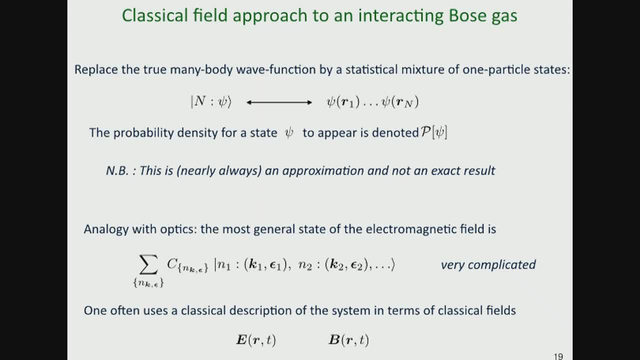 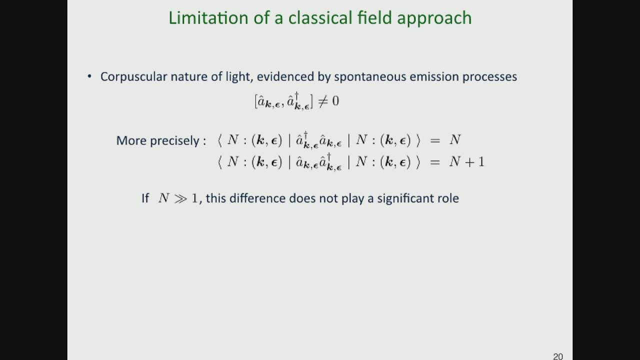 share the same side, but this side is a fluctuating object. what are the limits of such an approach? so, again, maybe a good way to see that is to come back to the electromagnetic field. when we do that, when we take a classical field approach, we neglect the fact that 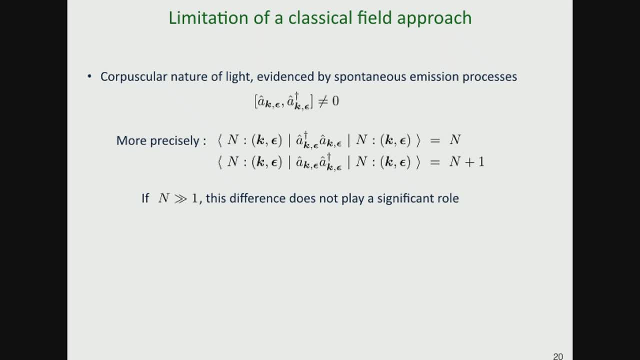 we have a set of elements of individual photons, so we neglect the corpuscular nature of light, and if you want to understand what a photon is, you have to look at, say, a spontaneous emission process where you have photons emitted one by one. so when are these processes relevant? 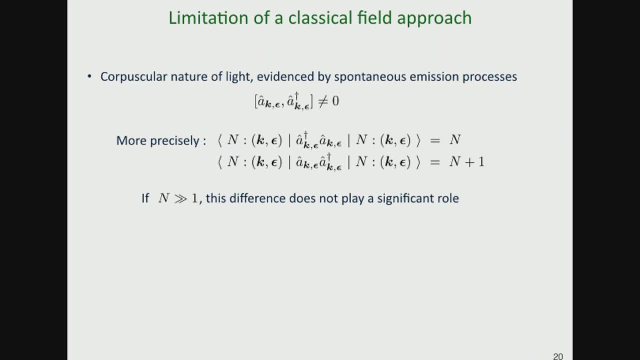 this spontaneous emission process. when will a classical field approach be bad? when will it be bad? when, actually, you do an experiment which is sensitive to the commutator between a and a dagger, which will tell you that it is not the same to take a a dagger. 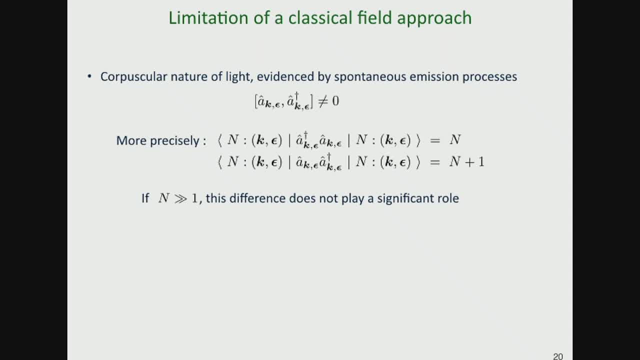 and if you look at what is the matrix element of a dagger, a and a a dagger, since this commutator is equal to one, this one will be equal to n, where n is the number of photons in the mode k, epsilon, and this one will be equal to n plus one. 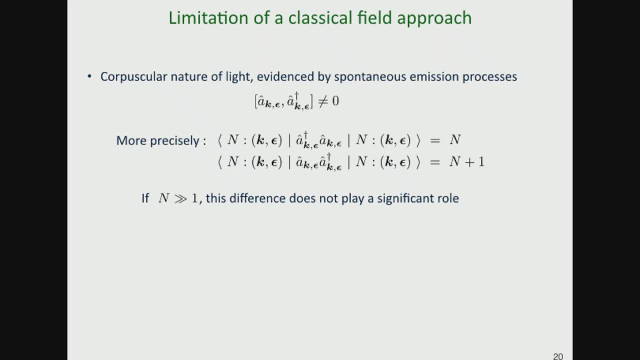 so if I have a mode which is heavily populated, if I have a number of photons n per mode which is very large compared to one, the difference between n and n plus one is not significant, whereas if I am doing something like spontaneous emission, a vacuum mode which is initially 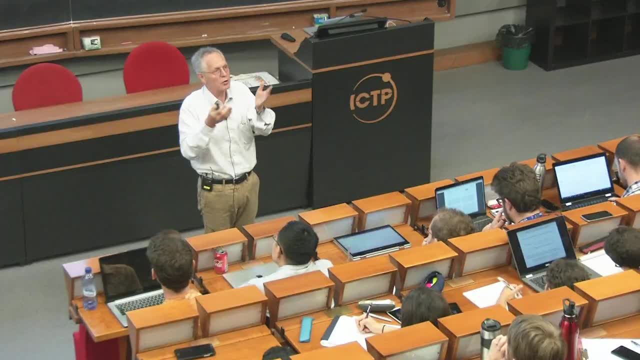 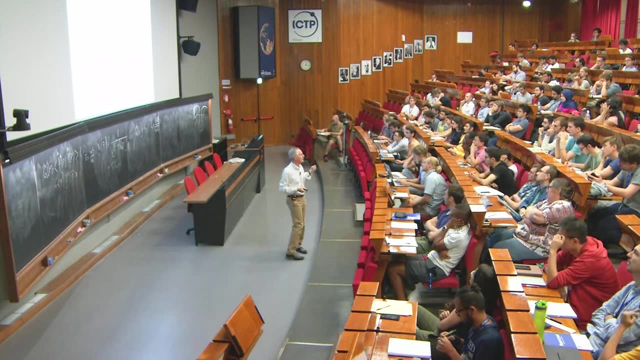 in the vacuum state and I emit a photon in it there. of course I cannot neglect the fact that the photons are quantized. so this classical field approach a priori will be valid if I have a large number of particles per mode of this matter: wave field. 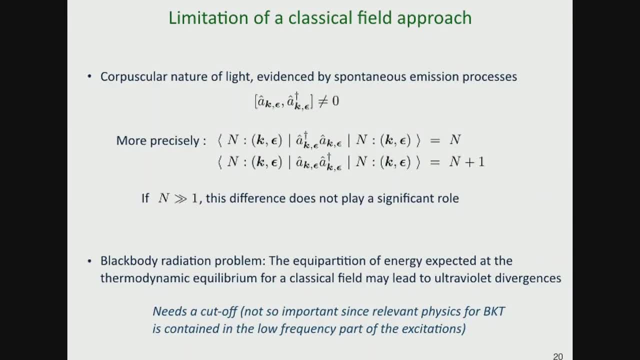 that I am going to introduce. another issue that you have when you use a classical field approach is the so called black body radiation problem, a famous problem of the 19th century. that is when you are doing classical field physics and you are looking at the thermal equilibrium. 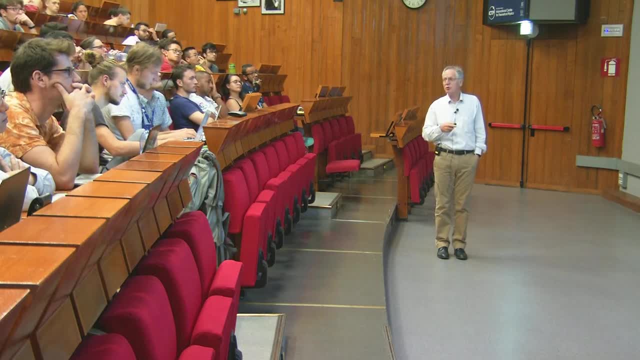 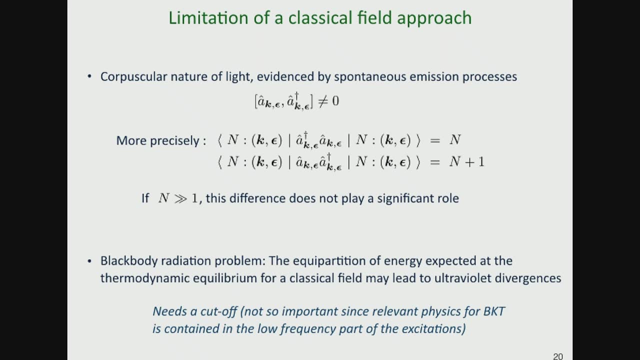 of a classical field, then you may have some ultraviolet divergences and therefore you need a cut off, that is, you need to not to consider frequencies which are very, very large. you have to put a cut off in your frequencies, otherwise you have divergences. 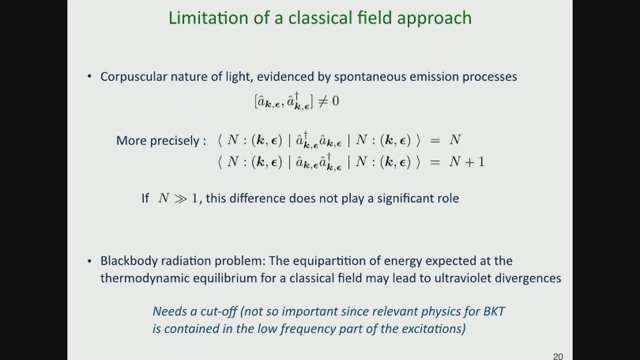 so here we will do that. it is not so important for us because, as we have seen, all the physics that Peierls introduced and what will come with BKT physics is a physics of, as I have explained, low momenta, low frequency. this is large distances. 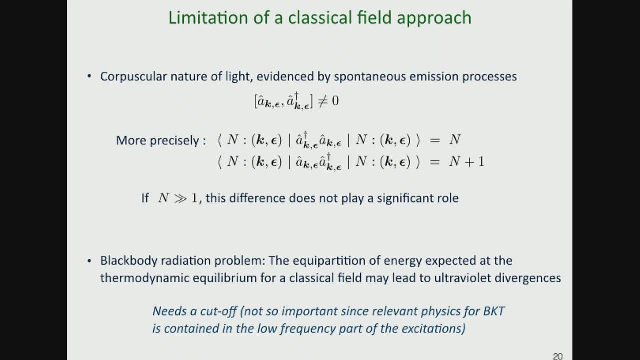 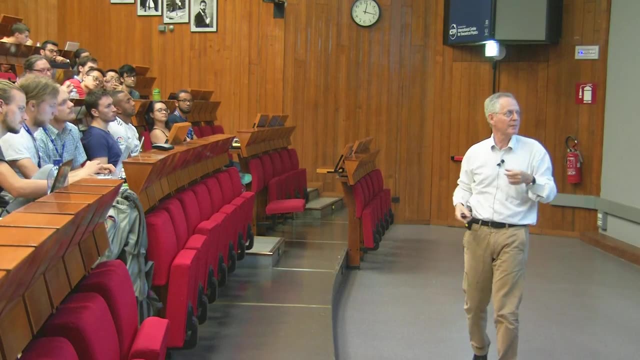 low momenta. so what happens at very large frequencies is ultraviolet. cut off is not so relevant for our physics, so we can put this cut off. it may mean some uncertainty on the prediction, but at least the main physics will still be present, because this physics belongs to. 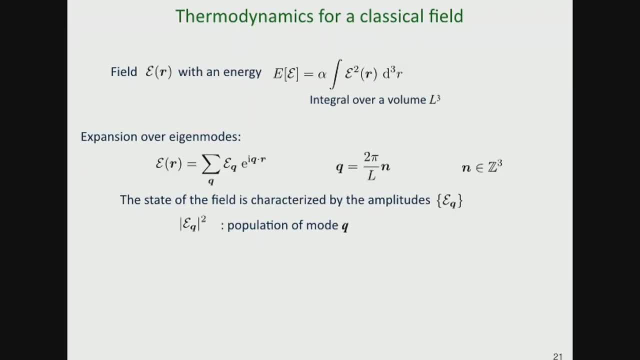 I would say infrared wavelengths and not ultraviolet wavelengths. so we have a field in thermal equilibrium at a finite temperature, T. so here I am doing it for the simplest field. I can think of a field like the electromagnetic field, where the energy I showed it with a field 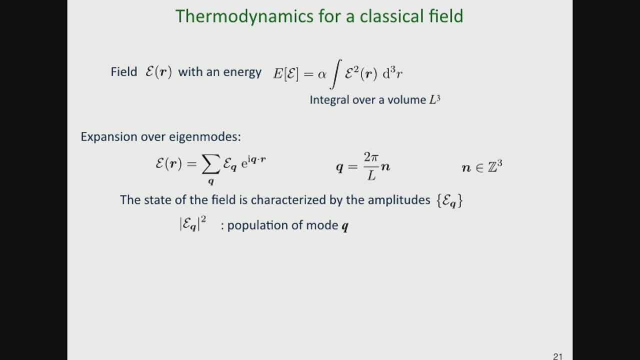 that I have written. by this E calligraphic the energy is promoted to E square, integrated over a volume, L cube. here I am doing it in 3D, but I could do the same in 2D or 1D. so again, the way to treat that. 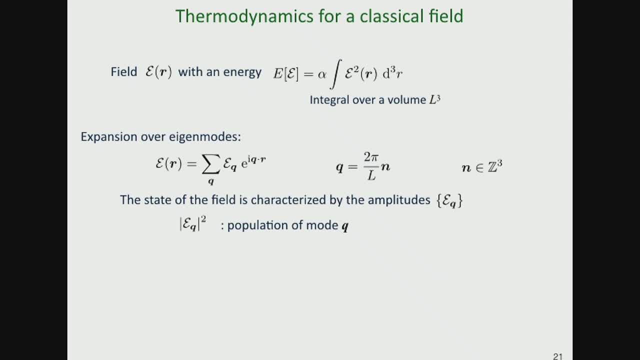 we are all independent from each other for this classic, very simple energy model, and so the state of the field is characterized by the amplitude E of Q, the Fourier component of this expansion, and E of Q square, is the proportion of the mode Q and the energy that was written here as an integral. 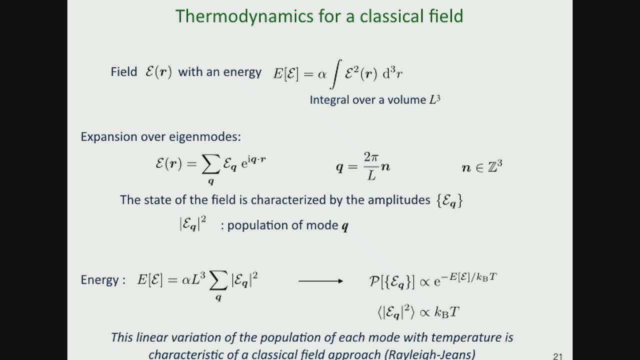 when I expand in Fourier space I get something which is alpha L cube. the integral of the whole volume times E, Q square. so the Fourier component square here and now. I just have to say that the probability to get a given realization for the field, that is, a given set of amplitudes, 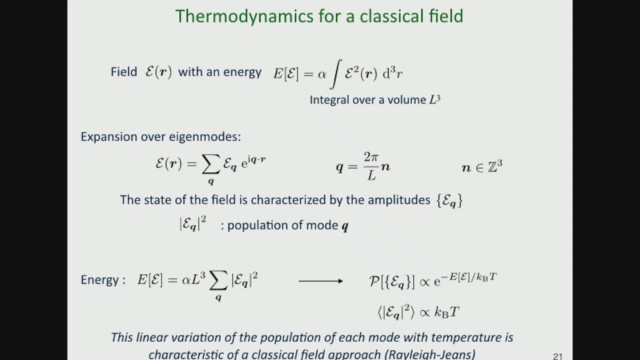 of E Q is just given by the Boltzmann weight exponential minus the energy over K B, T. and because E Q square, because the energy E of E is the sum of E Q square, I get that every E Q square has a thermal average which is K B, T. 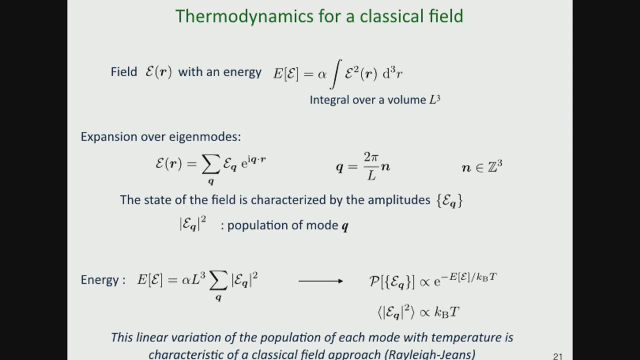 this is very similar to what I said before, but now it is at the level of the field, and this linear variation of the position of each mode is something that is very characteristic of a classical field approach, something you have probably seen when you have studied black body radiation. 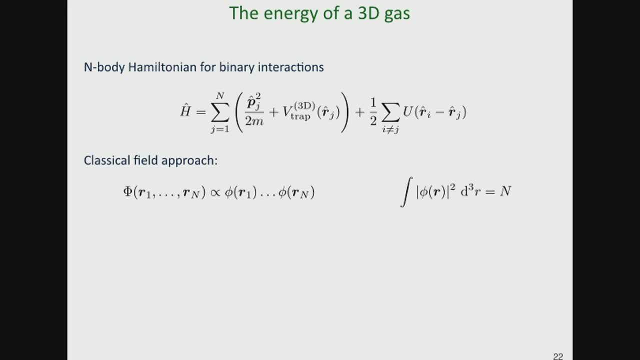 so we will do the same for our matter wave field. so let's see how it works with the matter wave field. so I take the energy of my gas, so this is my Hamiltonian I start with. so I have some kinetic energy, I have some trapping potential. 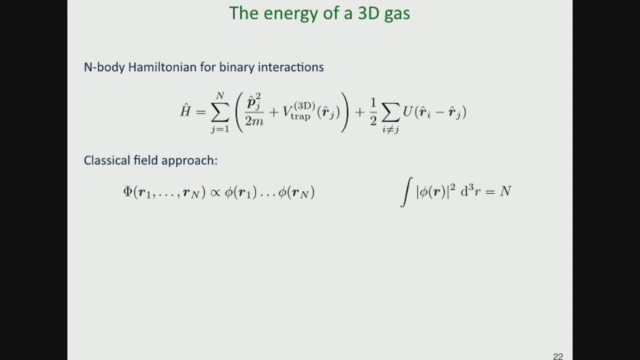 to hold the atoms and I have some interaction between the atom U of R I minus R J, with a one half here to avoid double counting. and in my classical field approach I am going to say that the wave function, macroscopic wave function of this system, psi of R1, R2, Rn. 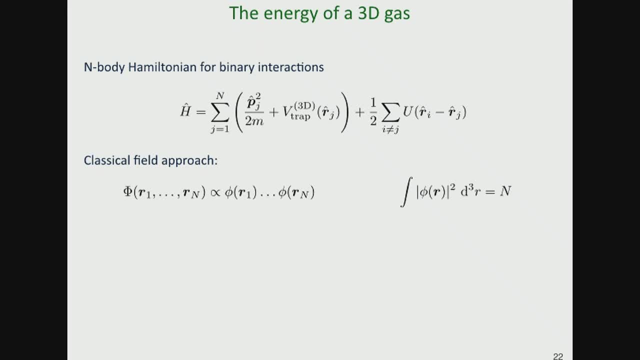 is simply a product state- little phi of R1, little phi of R2, little phi of Rn- and the normalization of phi is such that the integral of phi square over the volume is equal to phi square over the volume. so saying that, I get an energy. 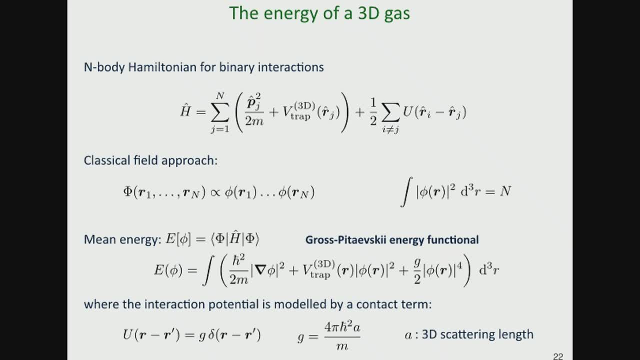 which depends on the field phi, which I will have to treat again as a fluctuating object, and this energy corresponds to the sum of all components that are here. so the pj square which are here will give me, you know that pj, in quantum mechanics, well, the momentum p is the gradient. 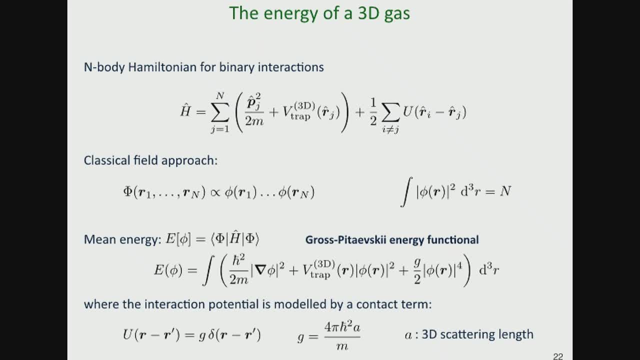 of the wave function. so the pj square, which are here, will give me h bar square over m, the trapping term here will give me v, trap of R phi square, and the interaction term here, u of R, i, R, i minus R, j, will be treated by a contact term. 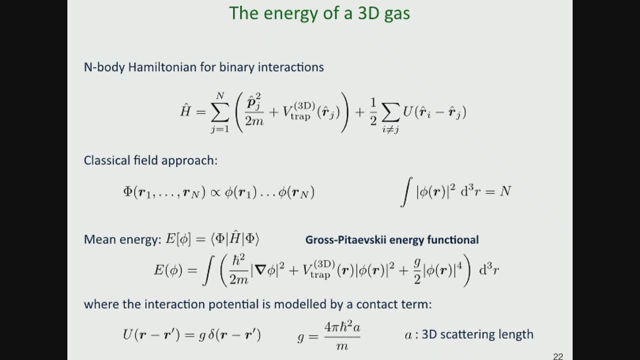 so it's an approximation, but it's a very good approximation for low energy physics for cold atoms. I treat this u of R minus R prime as a direct distribution. delta of R i. R minus R prime times some strength, little g. and then when I plug my ansatz here into this, 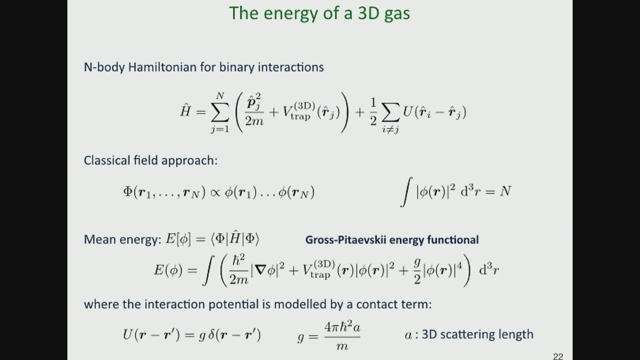 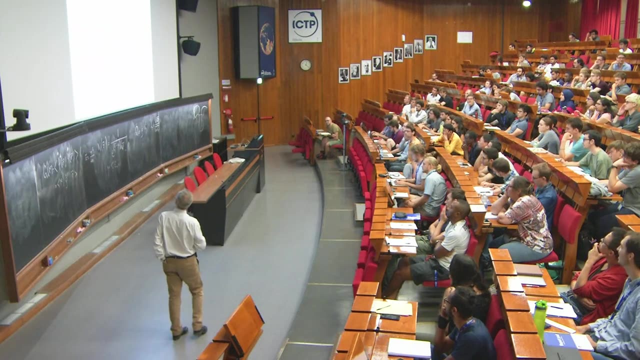 with this potential I get g over 2 phi 4. so a, here is the scattering length that Emmanuel already mentioned. so are there questions on that? no, you all know that. ok, so let's go now to 2D, and then probably I will stop. 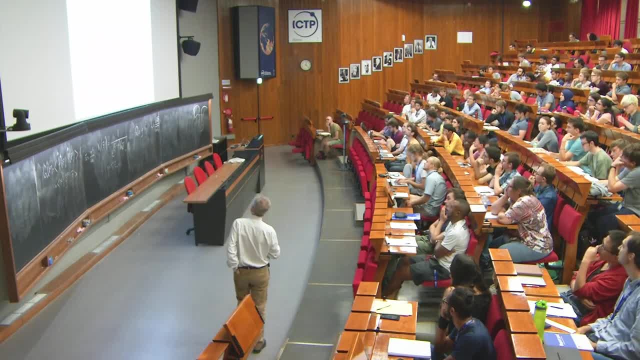 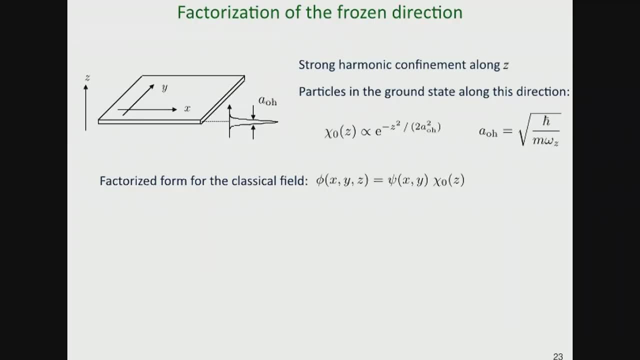 at this stage. so let's go to 2D. to go to 2D I have to freeze one direction of space. so I introduce a strong potential along the vertical direction and I assume that my particle only occupies the ground state of the vertical direction. so this ground state. 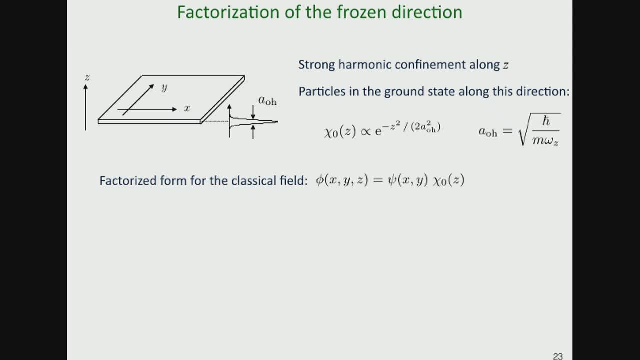 if I take, a harmonic potential is just a Gaussian distribution with a size given by the size of the harmonic oscillator, depending on the oscillation frequency in the potential along z. so the classical field that I was introducing before this phi of xyz is actually a factorized 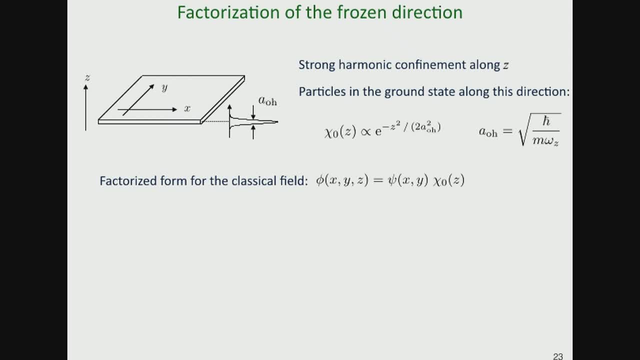 I have this chi zero of z, which tells me that I have frozen the vertical direction, so I know exactly the state of the particle for the vertical motion. and psi of xy is still a random field that I have to understand, and so when I plug the previous 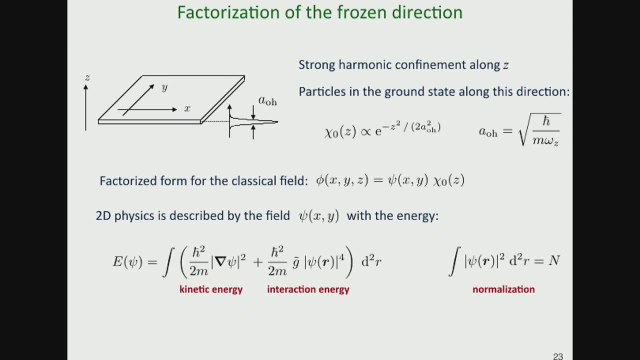 Gross-Petayevski ansatz that I had before into this. with this ansatz I get again a kinetic energy which corresponds to kinetic energy in the xy plane, which is the modulus square of the gradient of psi of xy. I assume that I have no more potential. 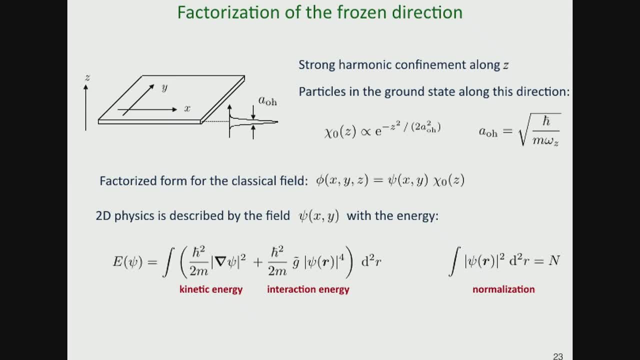 in the xy plane. so I have no potential energy, and the kinetic energy which was proportional to phi modulus to the 4, now is proportional to psi modulus to the 4, and I have introduced here some parameter g tilde, and this g tilde involves the previous scattering length. 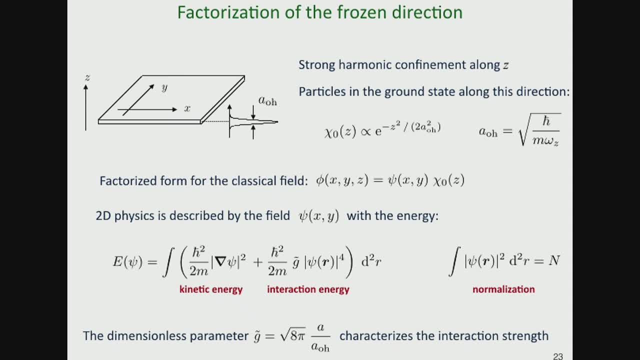 that I had before. and when I integrate over this chi zero, which is here, which is not complicated, I get little a divided by aOH. and what is quite remarkable in this expression here is that you see that I get the same h-bar square over 2m. 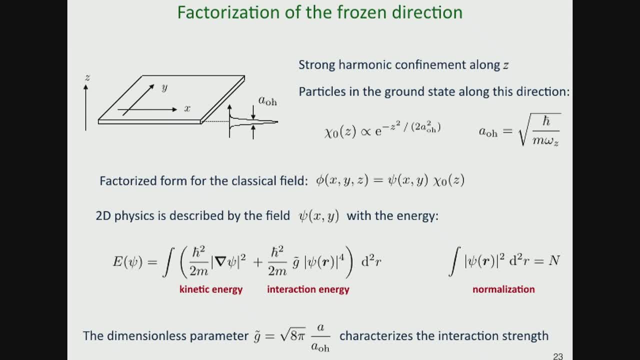 in front of the kinetic energy and the interaction energy times, this g tilde, which is a dimensionless parameter, and this is an important point I want to make. in two dimensions, at least within this classical field approach, the interactions are characterized by a dimensionless parameter, by contrast to 3D. 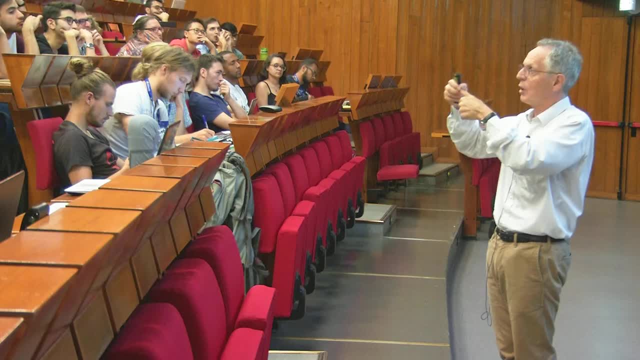 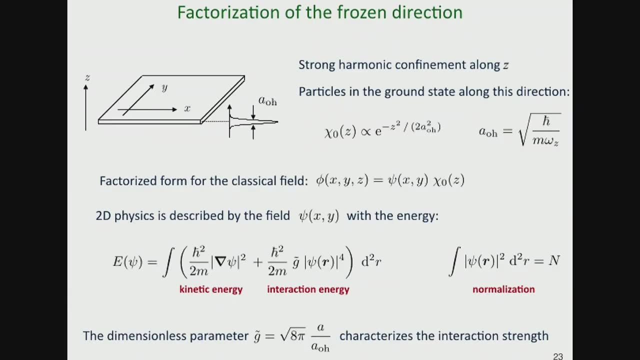 where interactions are characterized by a scattering length, so the number that characterizes them has a dimension. here it has no dimension. in practice it is a ratio between the scattering length and the size of the ground site of the Hamiltonian. but the fact that it is dimensionless 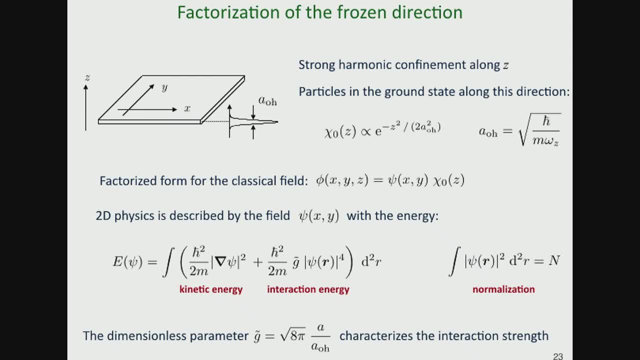 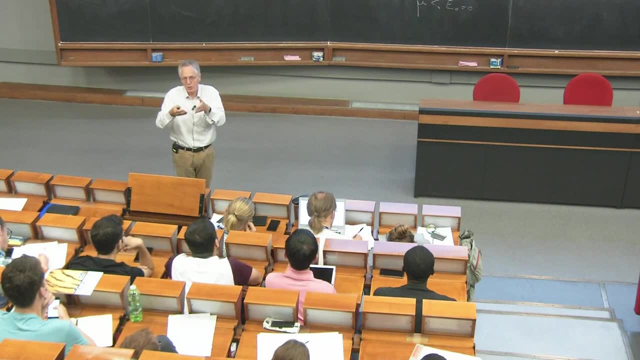 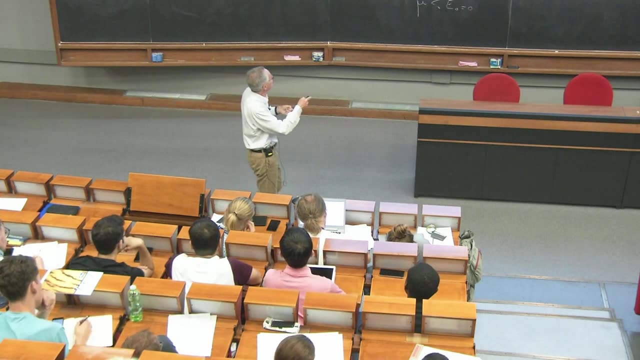 you will see tomorrow plays a very important role, because this is what gives the scaling variance of the 2D formalism, by contrast to 3D, where the interactions were introducing a length scale or an energy scale which comes with the interaction. the only thing I need to know. 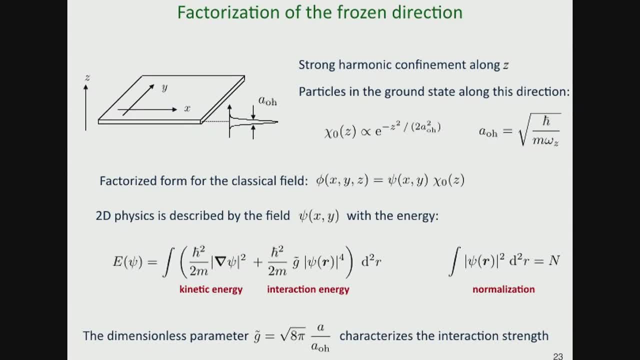 is the value of g tilde, and in a standard experiment it is between 0.1 to 1, and this is the only thing that has to be known about the 2D Bose gas, because this is a dimensionless parameter. okay, so what do you think? 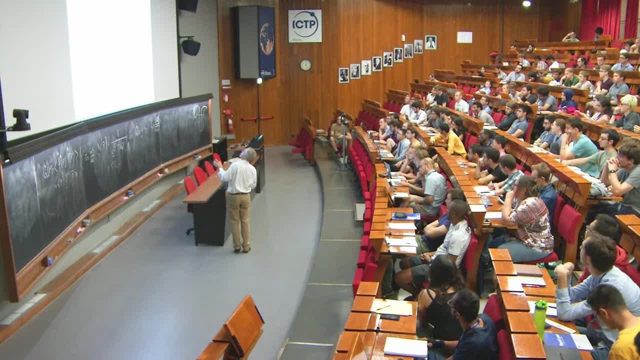 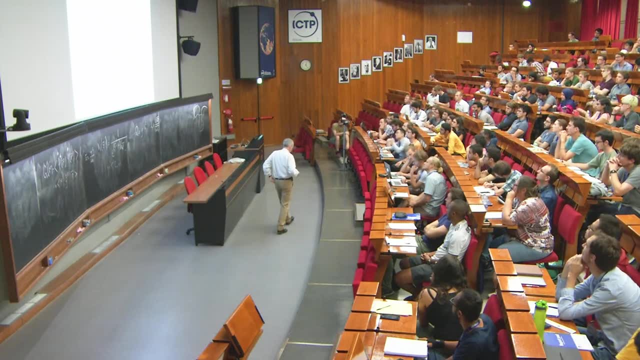 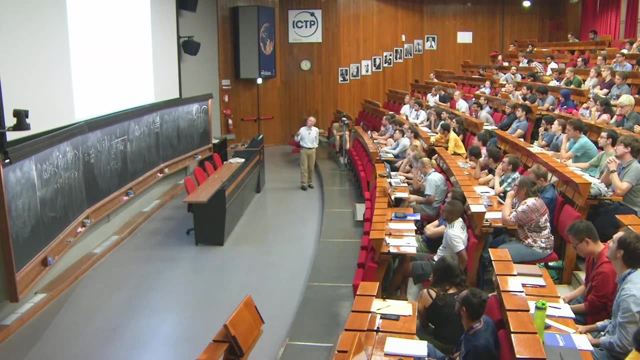 should I stop here or I can take questions. if you want, I can continue, but maybe I can just show this slide so that you can have lunch peacefully. you may wonder, when I am doing this classical field approximation, whether there is any quantum feature left in my problem. 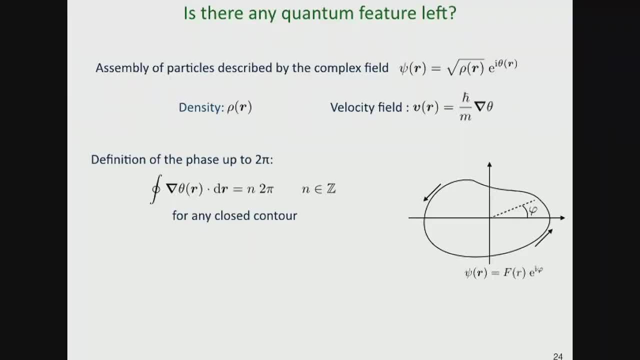 the fact that I have replaced all the quantum commutation relation by C numbers. are there any quantum feature left in the system? and the answer is yes. there is still something which is quantized in the problem, which is related precisely to the fact that we are using a classical field.